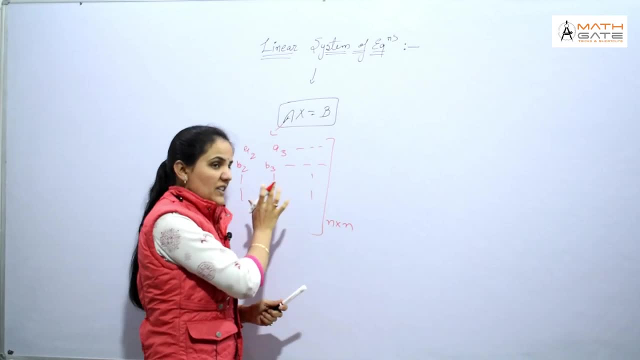 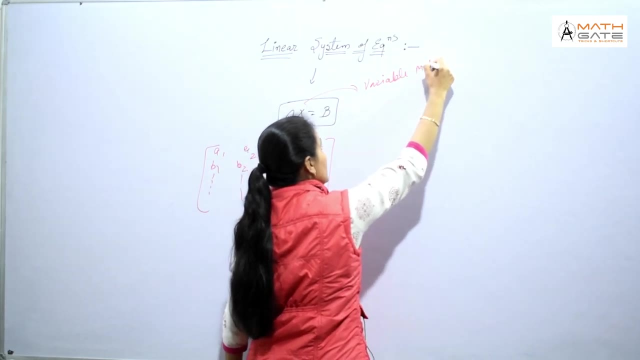 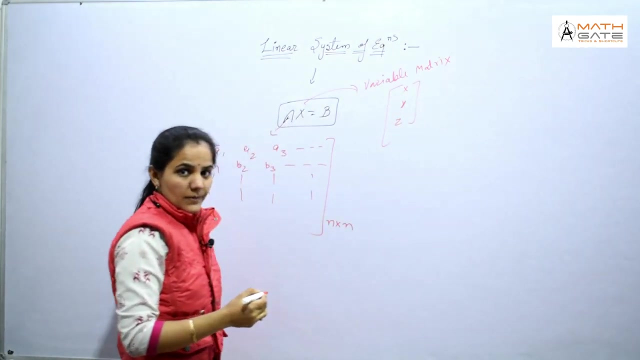 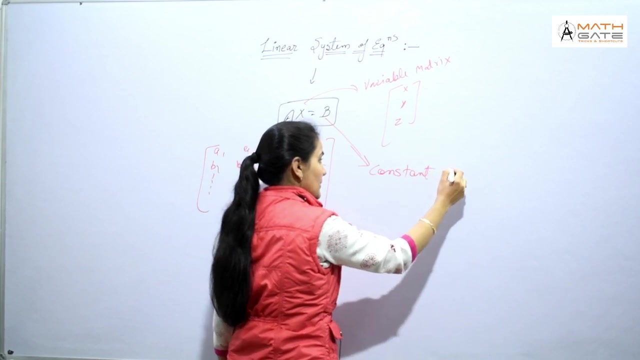 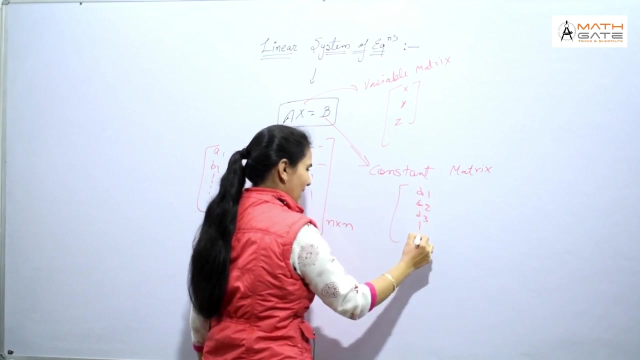 we can say: the matrix A is nothing but a coefficient matrix. X is what X is: a variable matrix, Variable matrix. or we can say: it is written in the form of X, Y or Z or X1,, X2, X3 and this B is a constant matrix. Constant matrix means D1, D2, D3 or any constant term. 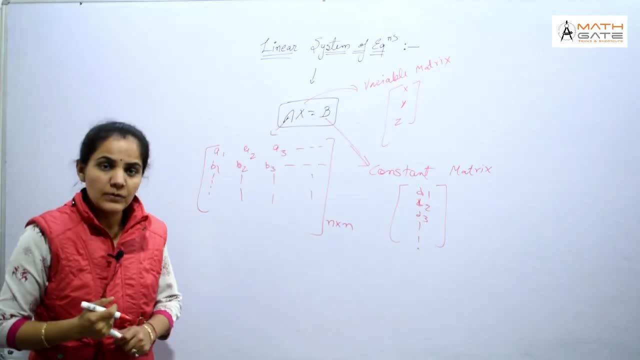 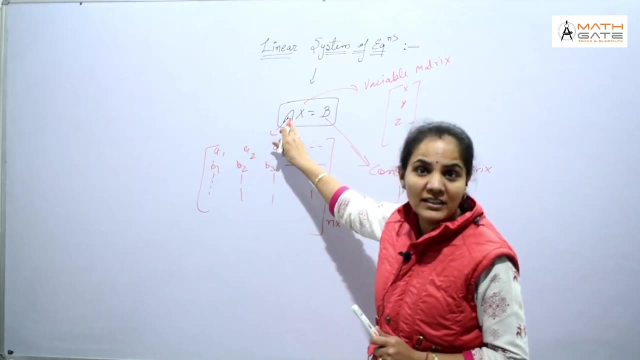 includes in this constant matrix B. So what AX is equals to B, AX is equals to B, X is equals to B, is matrix A, that is coefficient matrix, X variable matrix and B, that is constant matrix. What is the sum of these three? We can write these three in a form: 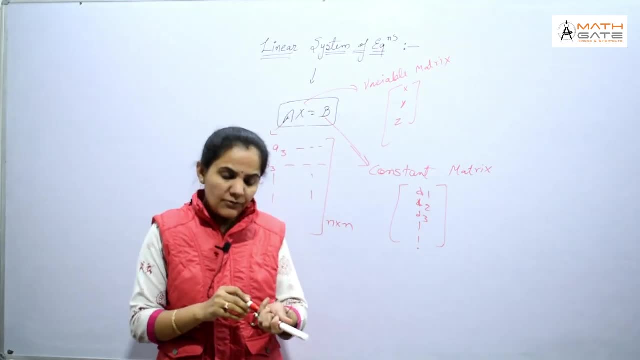 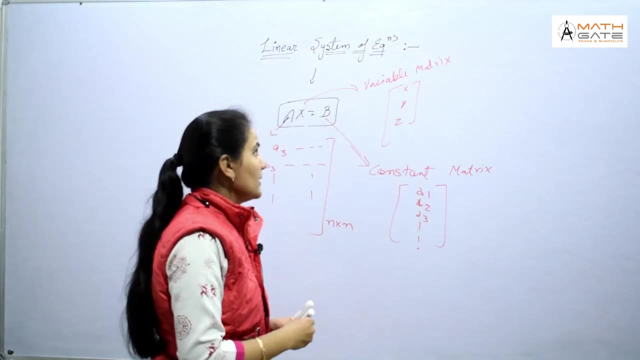 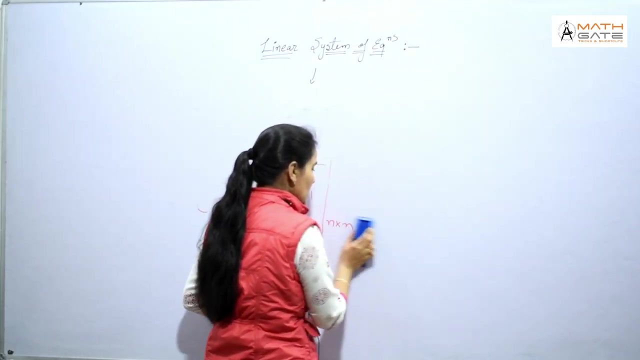 that is, AX is equals to B. Now, if we talk about the GET questions and we talk about what kind of question is made in GET, in AX is equals to B or in linear system of equation. So before that we have to discuss about the type of linear system of equation which comes. 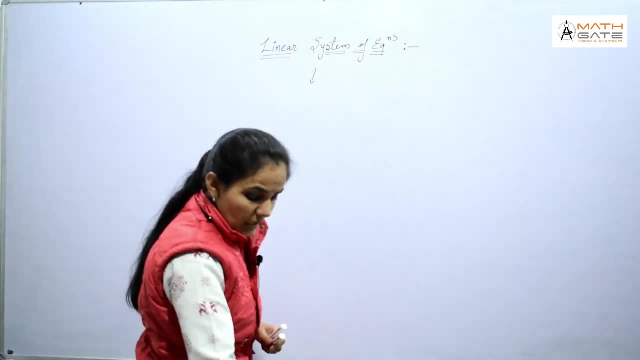 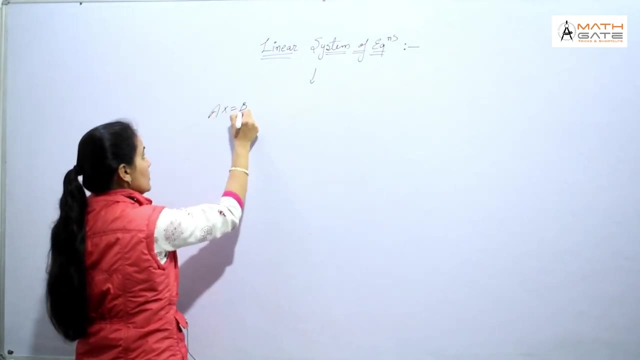 in GET examination. or we should say there are two types of linear system of equation which come in GET examination. So linear system of equation. the linear system of equation which is coming and which we are going to discuss is of two types. First, AX is equals. 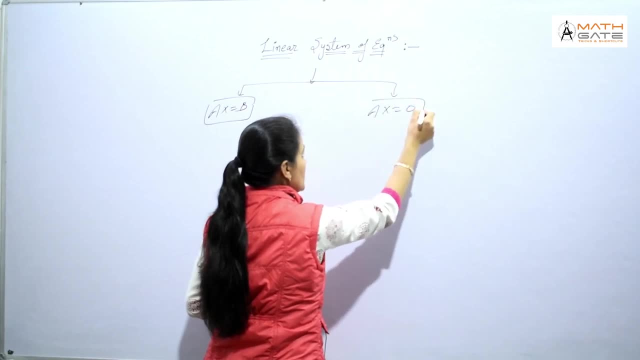 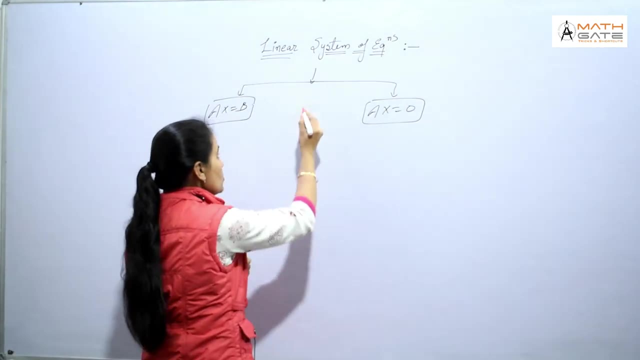 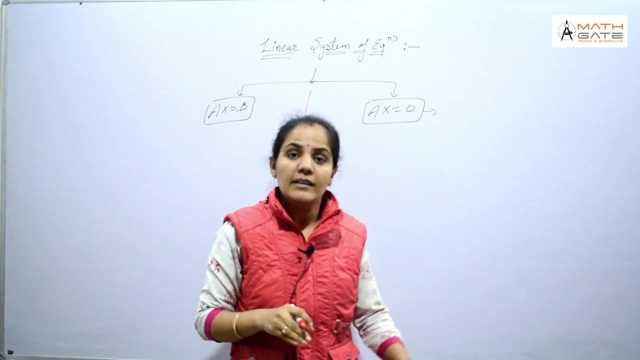 to B. and second we will discuss AX is equals to 0.. Here AX is equals to 0. we will discuss first and then we can discuss AX is equals to B. As I have said, AX is equals to 0 means what is 0? here Constant matrix is 0. So if the constant term of any system of equation 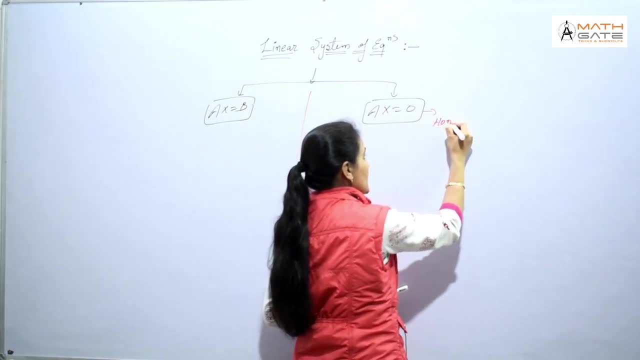 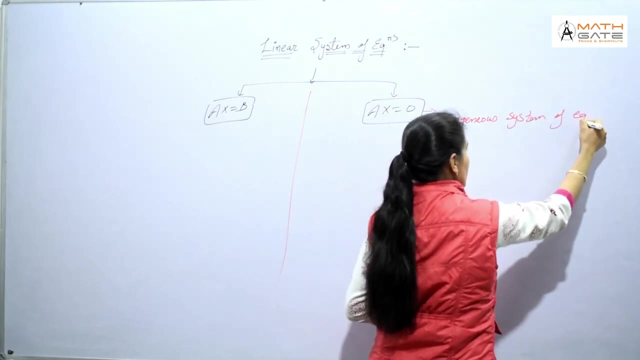 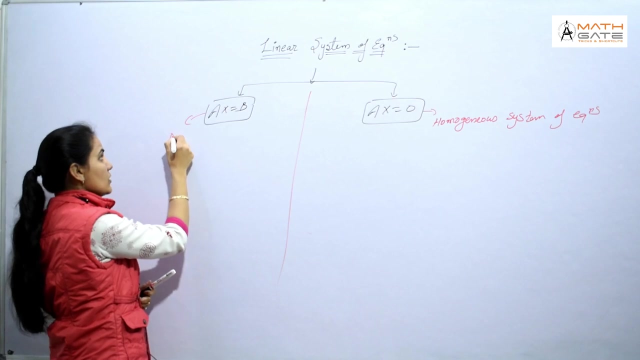 is 0, then what will become of that system of equation? It will become homogeneous, So it is a type of homogeneous system of equation. This is homogeneous system of equation. AX is equals to 0 and here constant term exists. It means what is this? We have non-homogeneous. 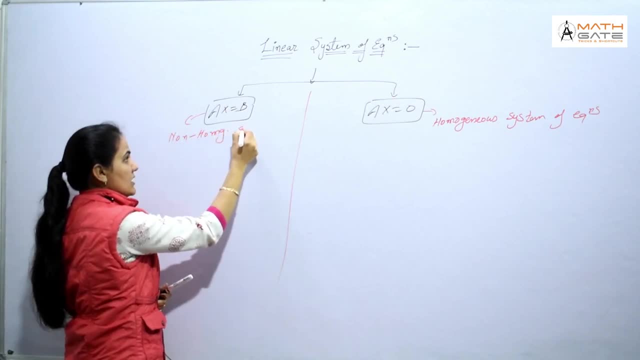 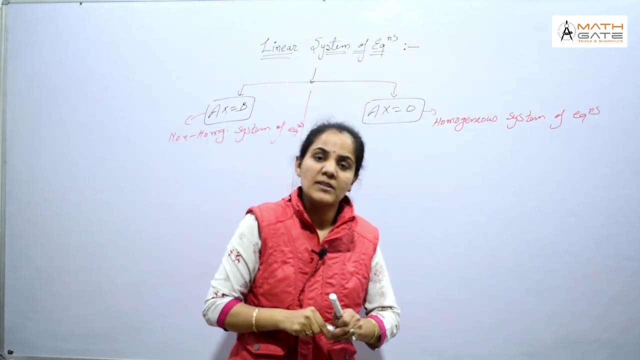 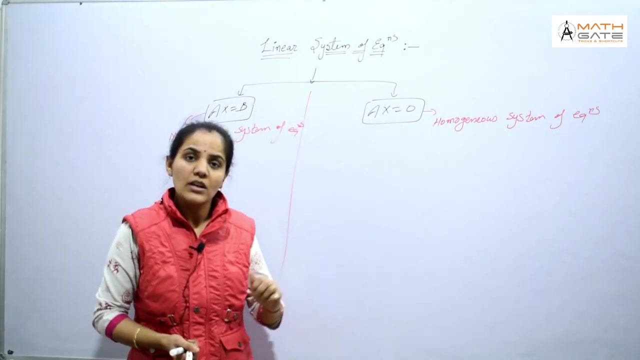 system of equation, Non-homogeneous system of equation. Okay, Now let us discuss one by one. First we will discuss AX is equals to 0 or homogeneous system of equation. Then we will discuss about AX is equals to B or non-homogeneous system of equation. Students- 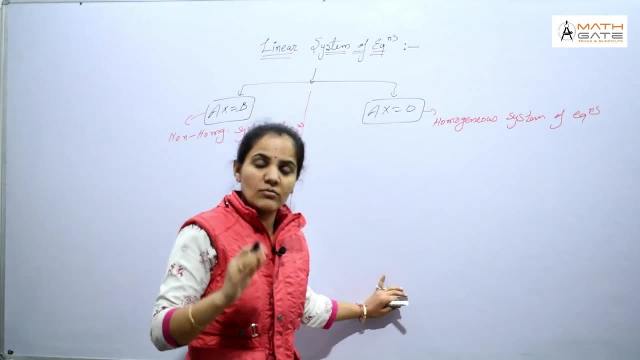 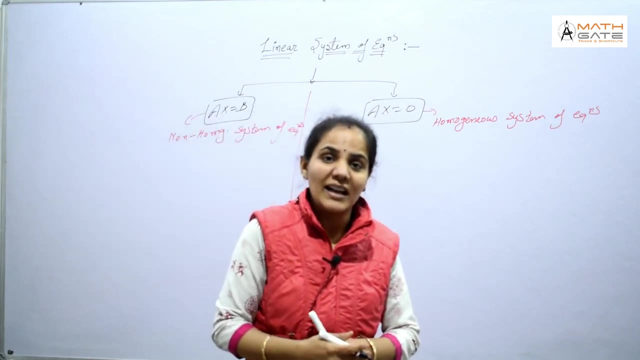 see. first of all, if we talk about homogeneous system of equation, then for this, if I have written like this: AX is equals to 0, what are we doing? What are we checking in linear system of equation? We are checking whether you go to homogeneous or non-homogeneous. 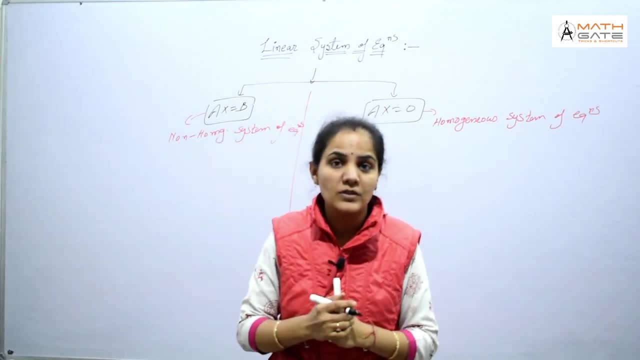 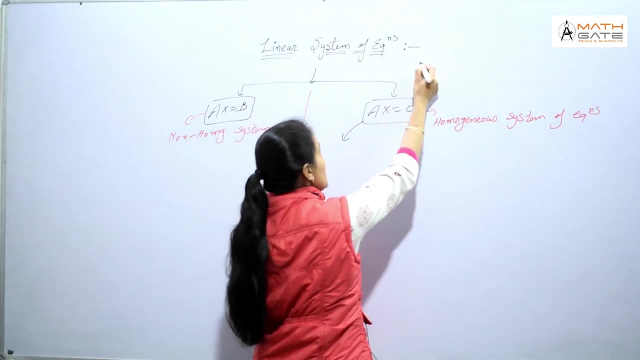 We are checking whether these two types of system of equation that I have written, or both, are linear system of equation. are they consistent or not? I have written a word here: Consistent These two system of equation? are they consistent or not? First, let us discuss. 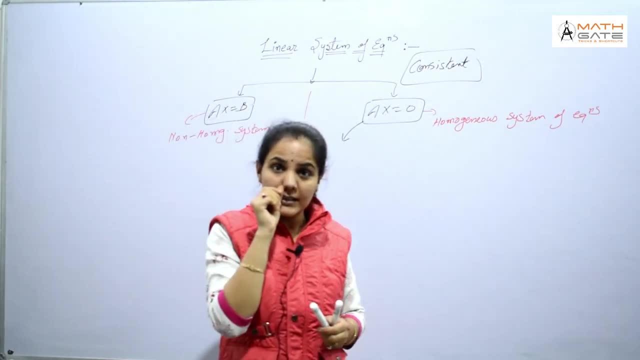 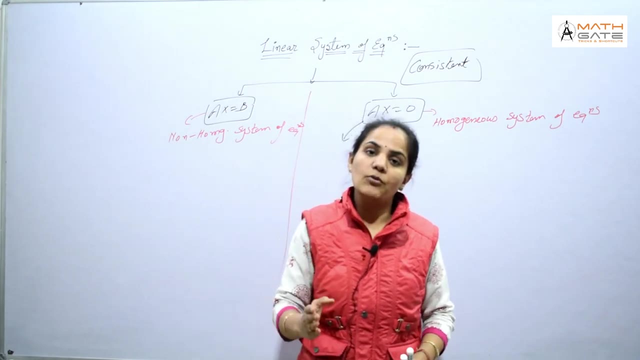 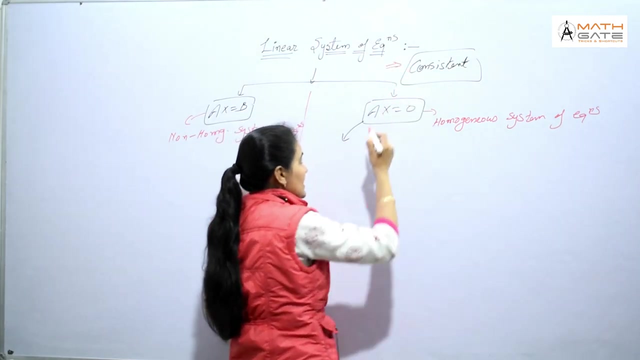 this Consistent means if in any system of equation at least one solution exists. If in any system of equation at least one solution exists, then that system of equation is said to be what Consistent system of equation? Okay, If the system of equation that you are 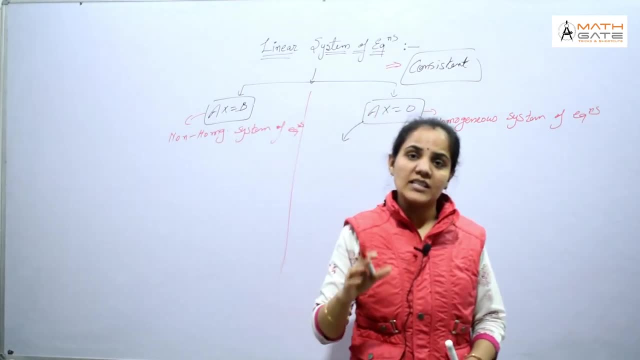 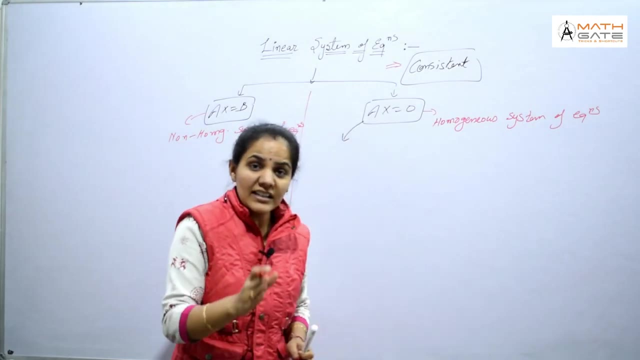 talking about whether it is homogeneous or non-homogeneous, then that think of it as If there is at least one solution in it, then it will be called consistent, But if there is not a single solution in that system of equation, then it will be called inconsistent system of equation. 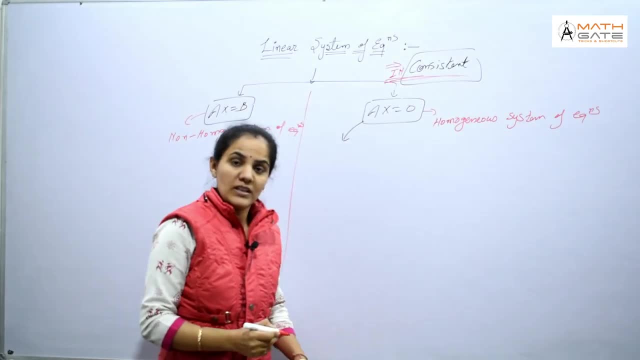 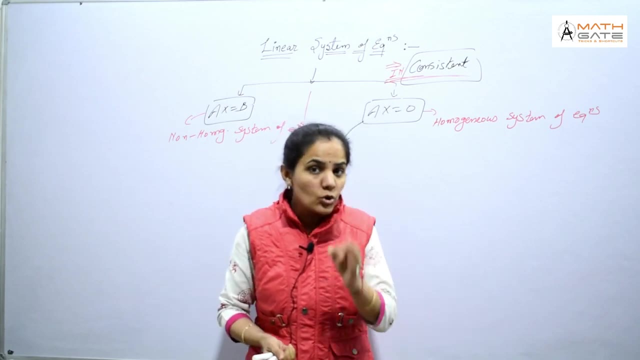 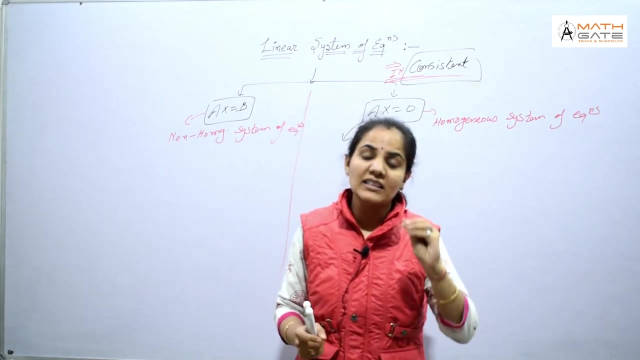 It will become inconsistent system of equation. So we are going to check here what we have already discussed in rank of matrix: Why do we find out the rank or why we find rank? The answer to that is for finding the type of system of equation which you are discussing. 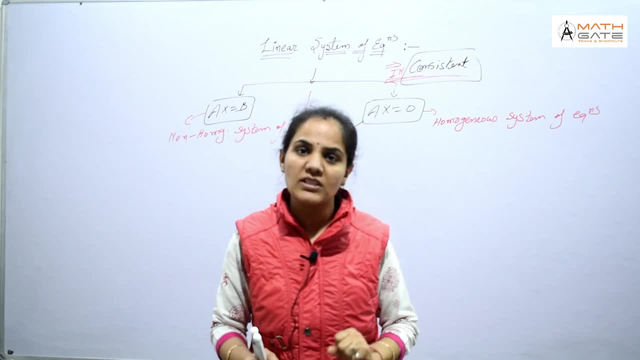 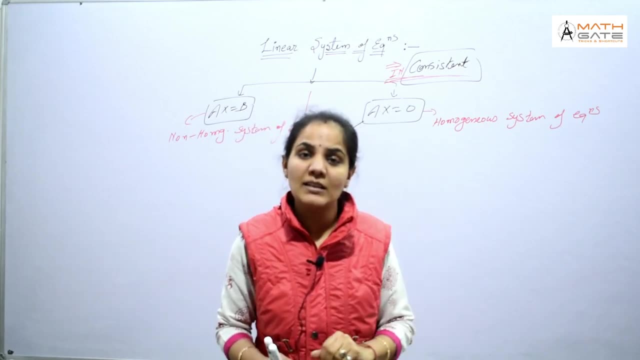 for finding the type of solution for that particular system of equation which we are talking about Means. if I talk about homogeneous, then for homogeneous, what I have to see is its rank. Whatever system of equation or whatever matrix is here, we will check its rank. 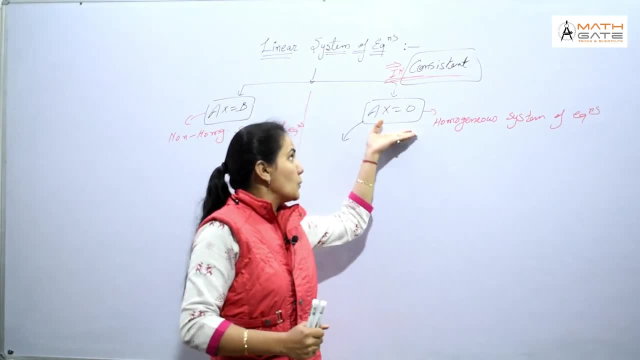 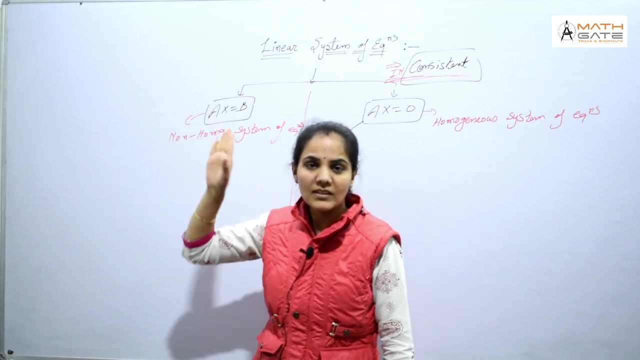 To check its rank. you will get the output from that. whether your system is consistent or not, Same with that, Ax is consistent. Ax is equal to b concept. Here you have to check the rank of matrix. Whatever matrix is given to you, you will check its rank. 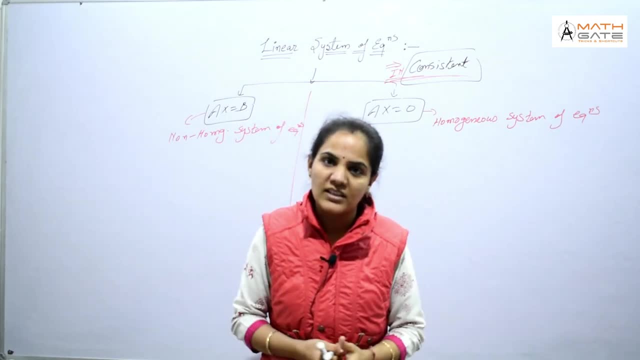 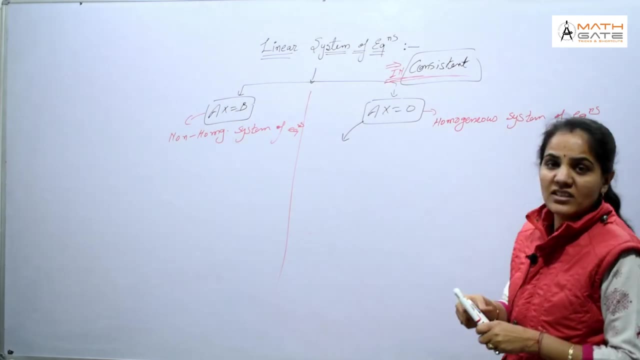 If that system is consistent, then at least one solution will come out. If not, then it will not come out. Okay, Now we will discuss this a little deeper. First of all, let's talk about homogeneous system of equation students. 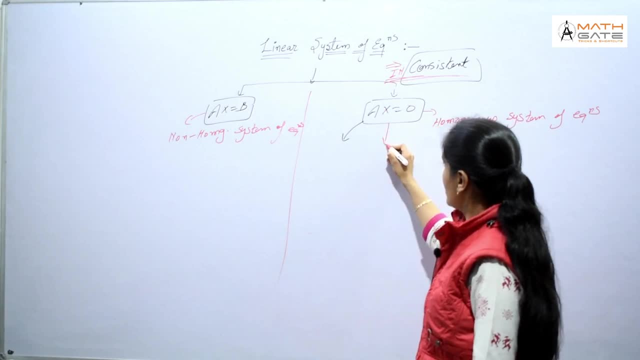 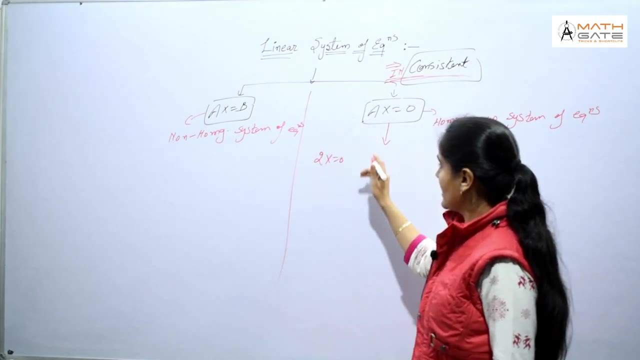 See, if we talk about homogeneous system of equation, what happens in it? Ax is equal to 0.. So if I write it like this, 2x is equal to 0.. Suppose I write it like this: 2x is equal to 0.. 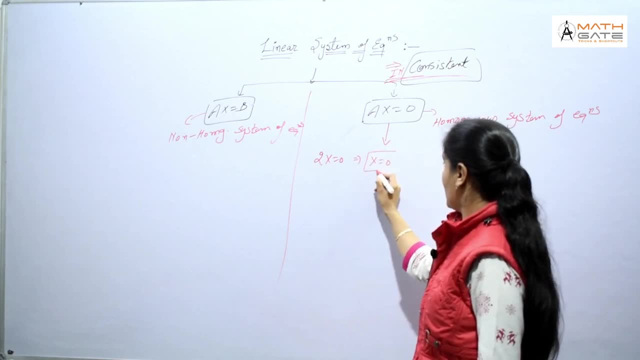 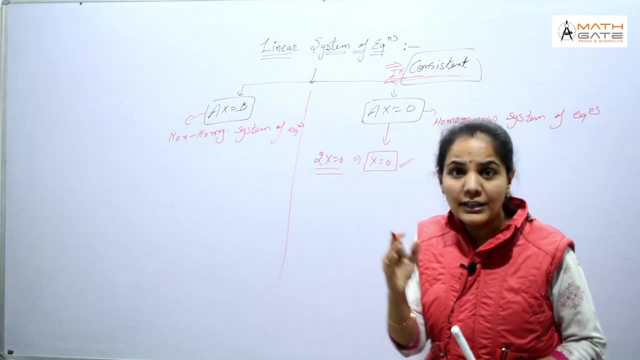 So every student from you can tell me that ma'am, 2x is equal to 0. It implies x is equal to 0 always. It means if 2x is equal to 0, I have an equation. So x is equal to 0, what will be its solution? 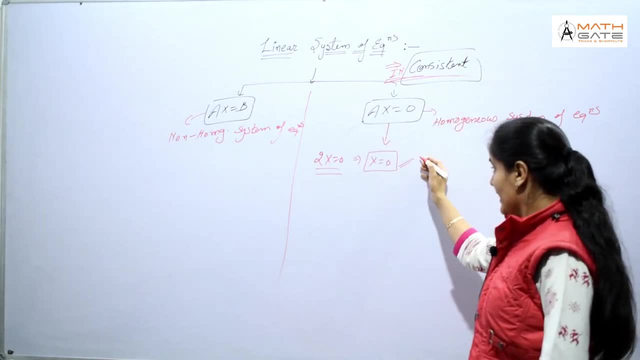 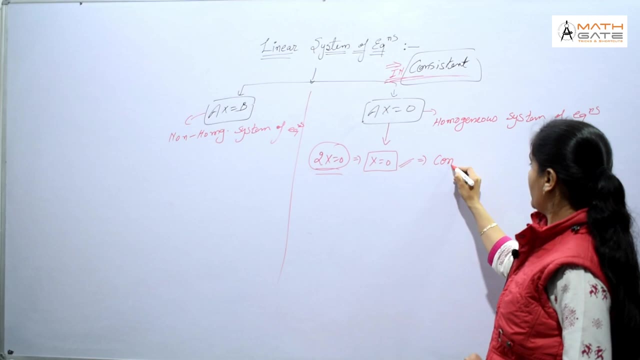 It will always happen. It will happen every time. Right? If x is equal to 0, it has a solution. So what will happen? What does it mean? This 2x is equal to 0 system will always be called. 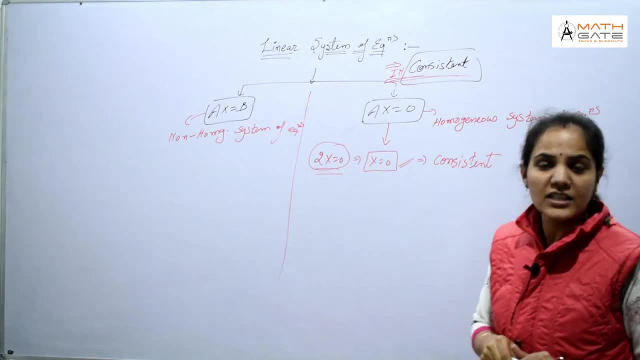 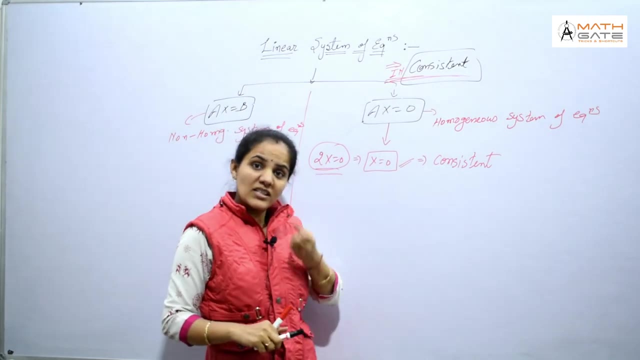 It will always be called Consistent system. If the solution of this 2x is equal to 0 is x is equal to 0, then this 2x is equal to 0 system will be called consistent Same with the given x is equal to 0.. 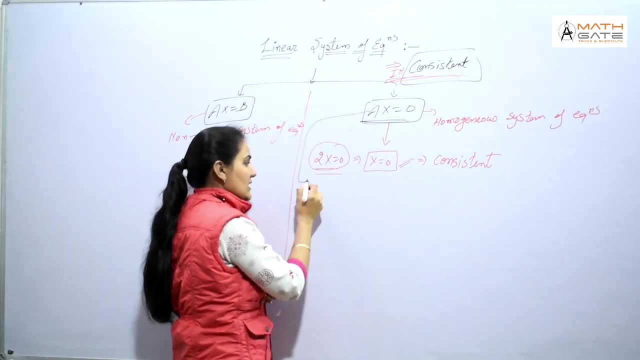 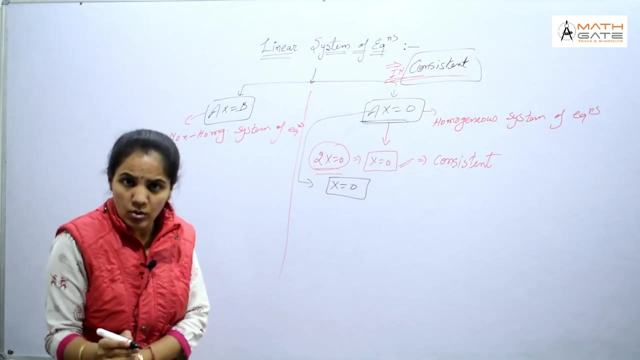 We are going to talk about this in that too. If this is x is equal to 0, then it is going to be sure, here, x is equal to 0,. what will be its solution? It will always happen. It will happen every time. 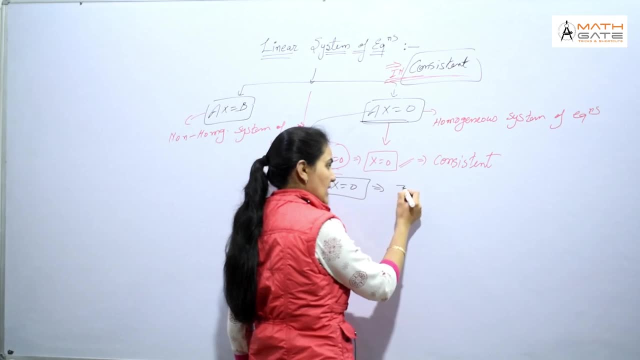 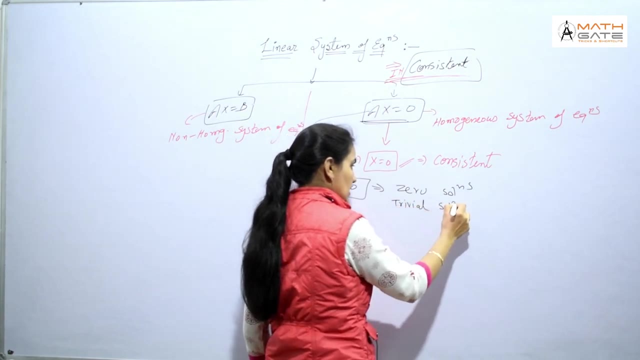 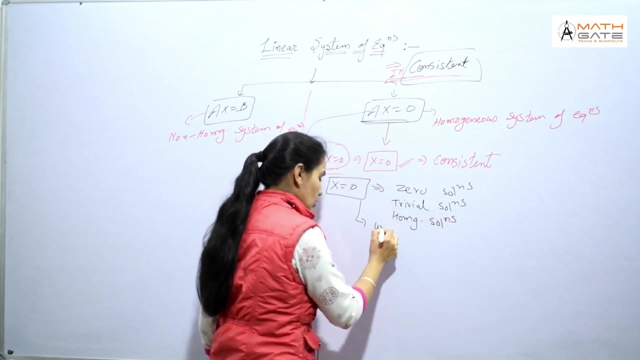 Right, And what will happen? We call this: x is equal to 0, zero solution, And we call this trivial solution And we call this homogeneous solution. Right, And in many books it is also written as unique solution. So we can say: if x is equal to 0 is my system of equations, then clearly it is visible that 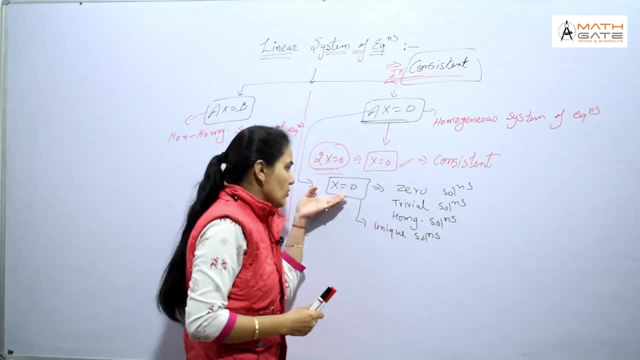 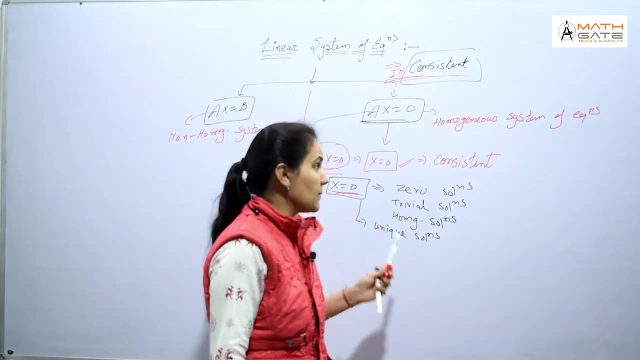 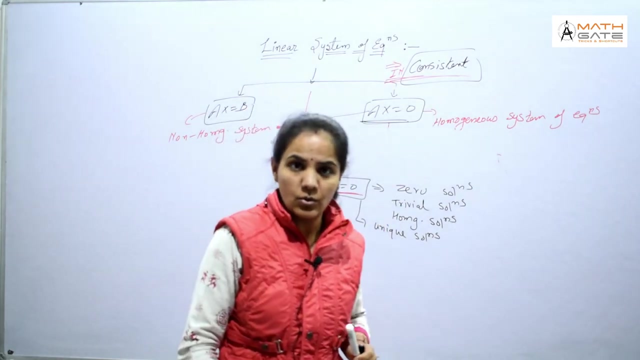 x is equal to 0, this system will always have a solution. If X is equal to 0, it means AX is equal to 0. system is always consistent. If AX is equal to 0, it means AX is equal to 0. solution is always consistent. 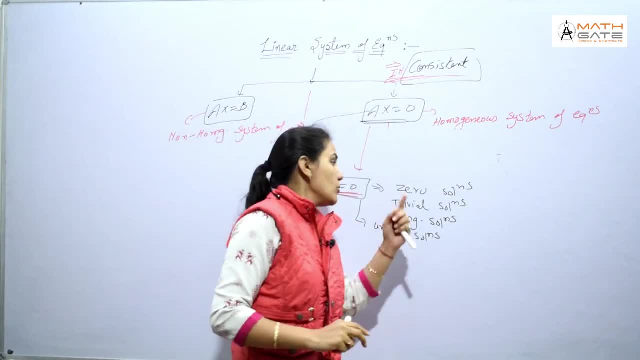 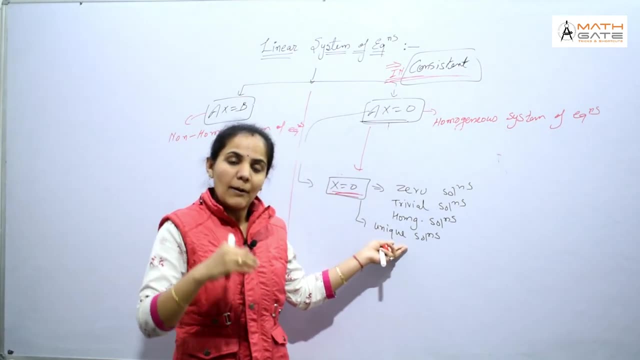 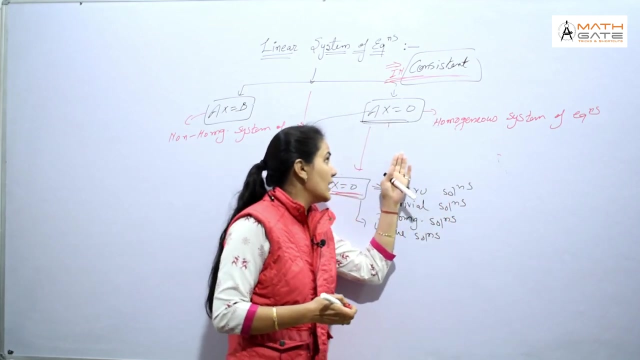 This X is equal to 0 can be called zero solution, This can be called tribal solution, This can be called homogeneous solution And this can be called unique solution. Now, if I want to find out that the given system of equation that we are talking about is AX is equal to 0. 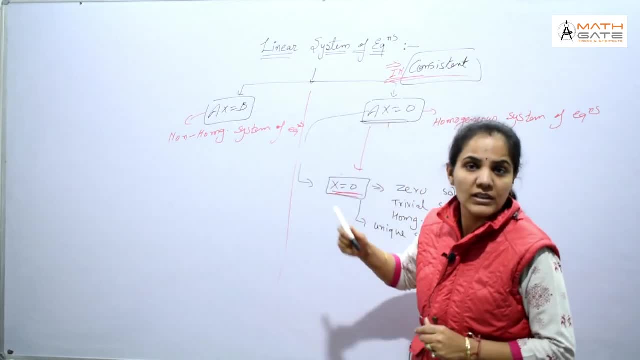 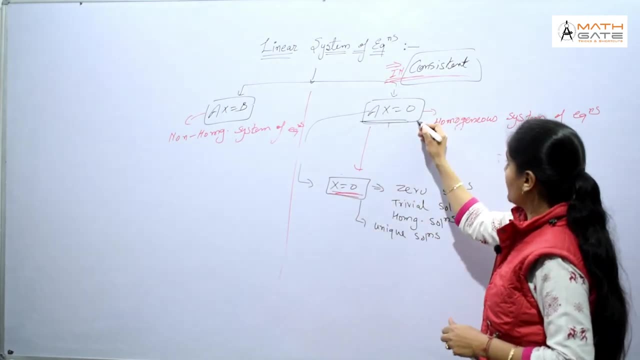 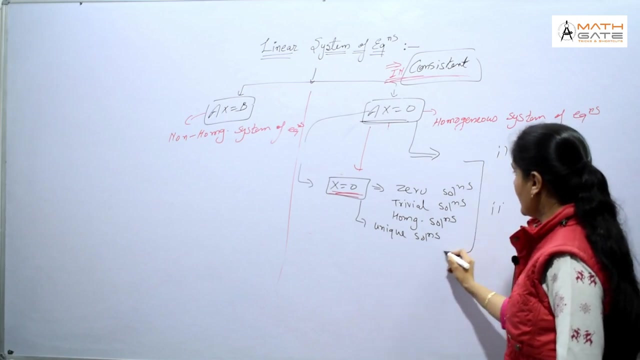 Is there any other solution in this system of equation other than AX is equal to 0?? If you want to know whether there is any other solution in this or not, then we will come to the concept that we discussed earlier. We will come to the concept of rank. 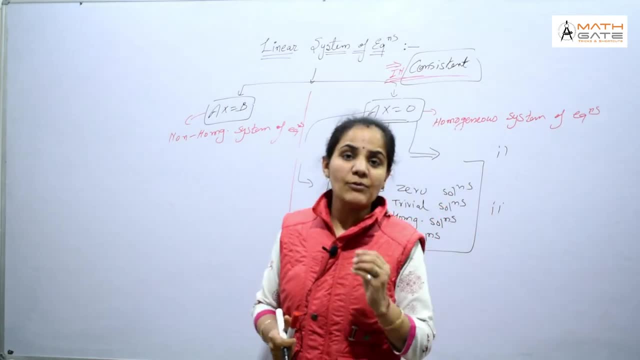 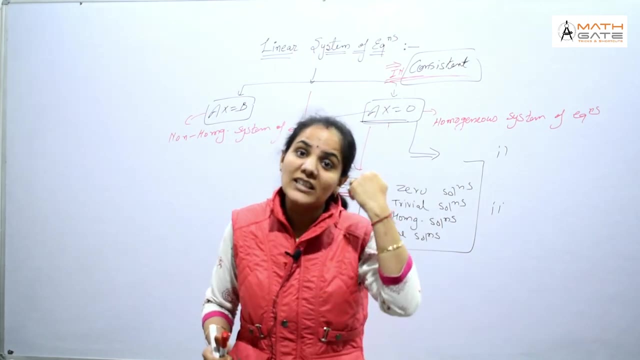 Because we find out the rank. that is why we find out that, whether the given system of equation has a solution or not, If there is, then how many solutions are there? Is it 1,, 2, or more than 1?? 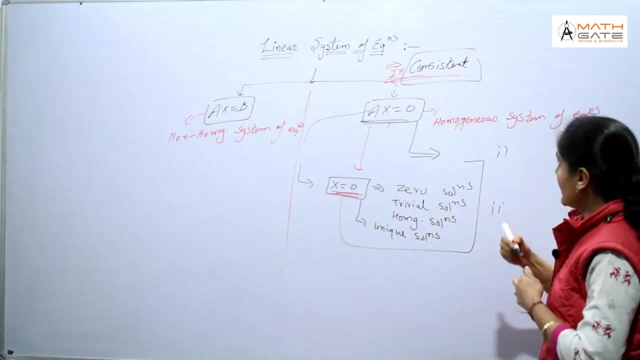 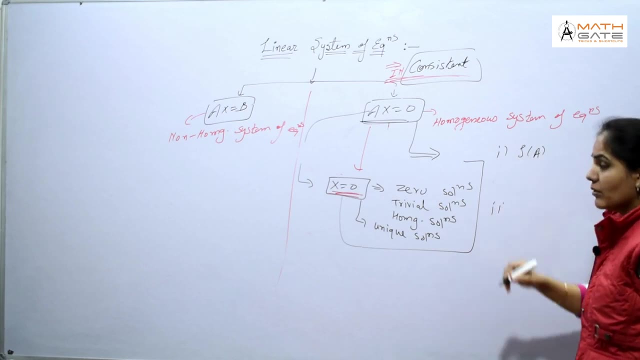 How many solutions are there? Okay, So that aspect. first of all, we will find out the rank of matrix A in this system of equation. AX is equal to 0.. If the rank of matrix A is equal to the number of unknowns, 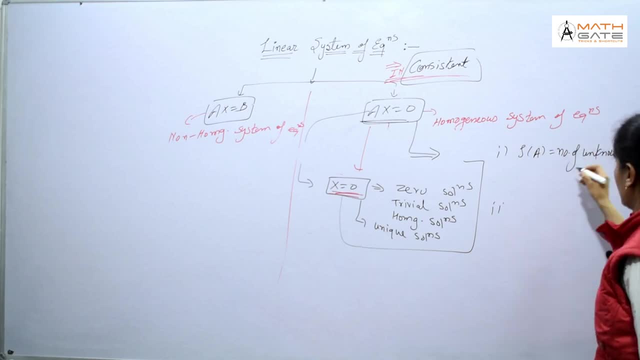 which is given to you. then you will find out the rank of A in the given system of equation, And the rank of A is equal to the number of unknowns. The number of unknowns means the variable. The variable means X, Y, Z. 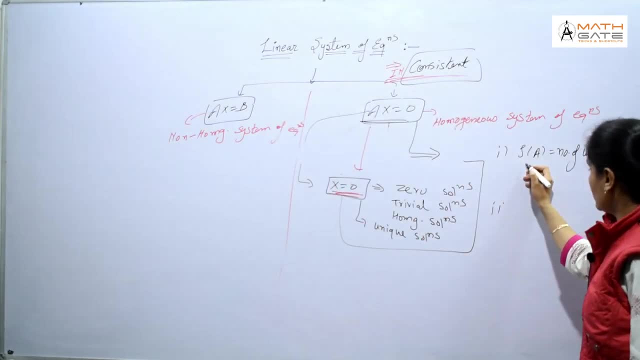 Which we are talking about. Okay, If the rank of A is equal to the number of unknowns, then you will clearly say that the solution of this given system of equation is going to be unique solution. What does this mean? We have already discussed the unique. 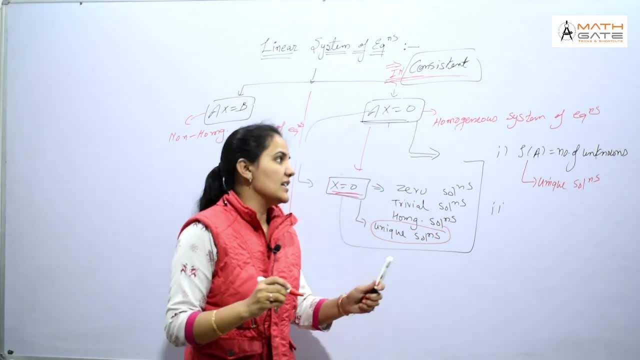 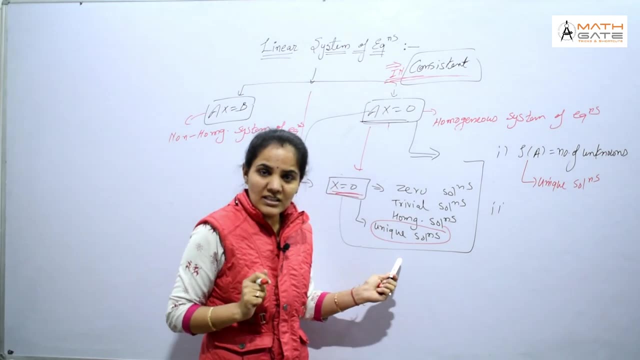 That means if for the system of equation AX is equal to 0, what do we have If the rank of A is equal to the number of unknowns? it means that for this only the unique solution will exist. We can call that unique as zero solution. 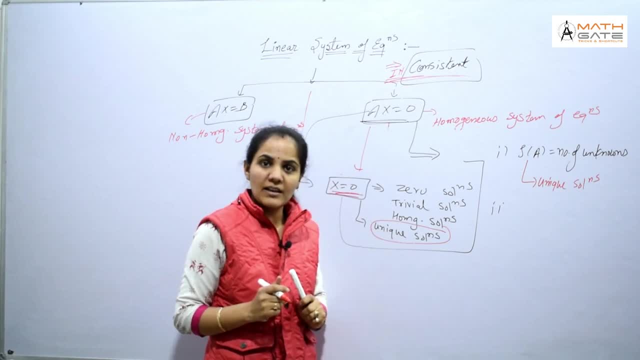 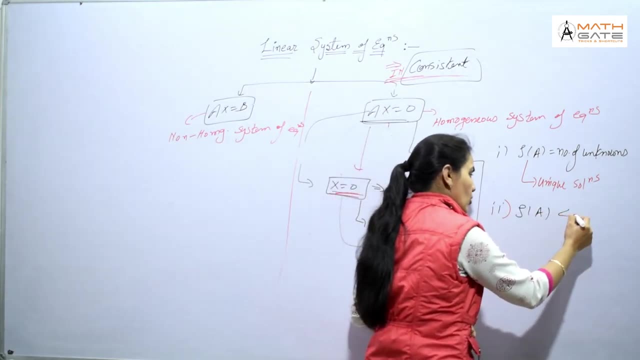 we can call it tribal, and what else can we call it? We can call it homogenous solution. Okay, Now if we discuss the second case, we have discussed that. I have found out the rank of A, and what is that? 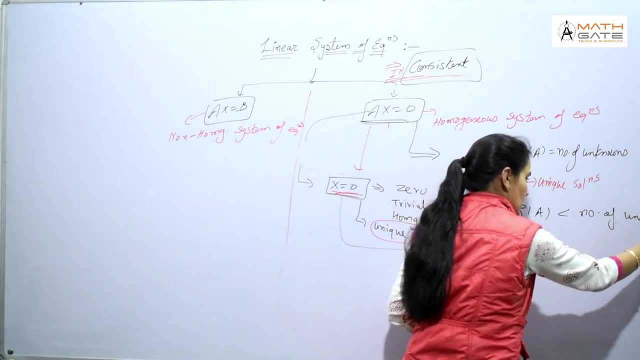 It is less than the number of unknowns. If we have found out the rank of A in this, and what is that? It is less than the number of unknowns. Suppose I have the rank of 2, and the number of unknowns is 3.. 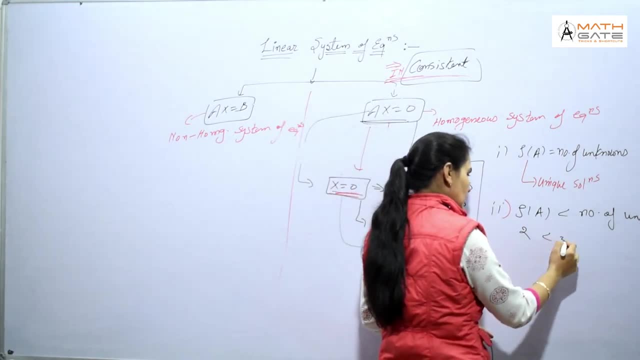 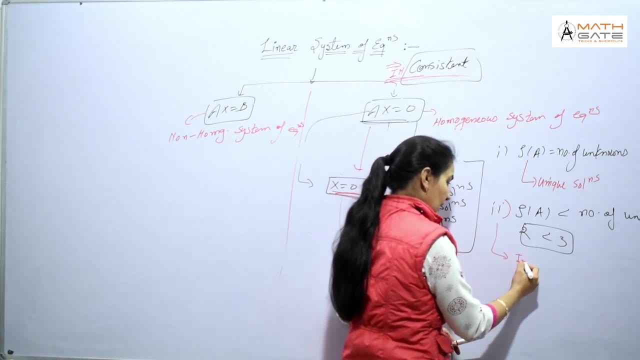 It means x, y, z, So 2 is less than 2, 3.. If you find such a concept then you will see, students, that this given system of equation, it has infinite number of solutions. It means there will be more than one solution. 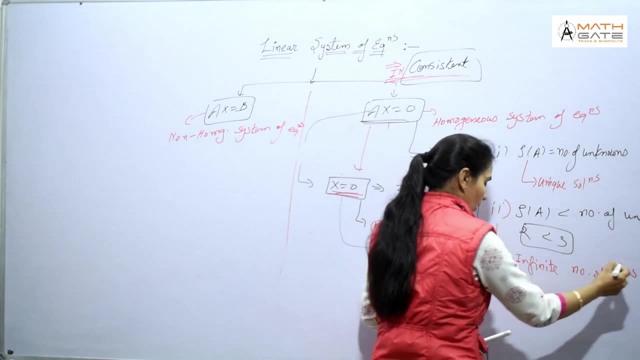 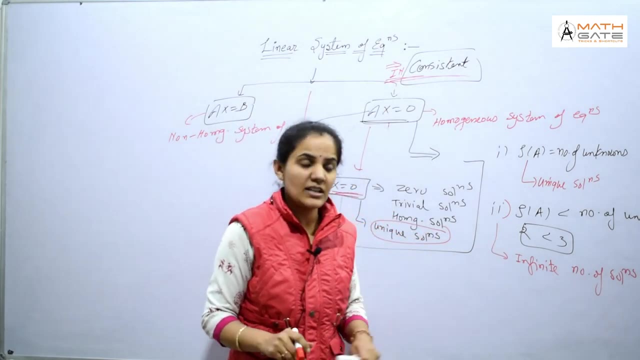 There will be infinite number of solutions. There will be more than one solution. There will be infinite number of solutions. Okay, For what? When you have the rank of A less than the number of unknowns, What will come from the number of unknowns? 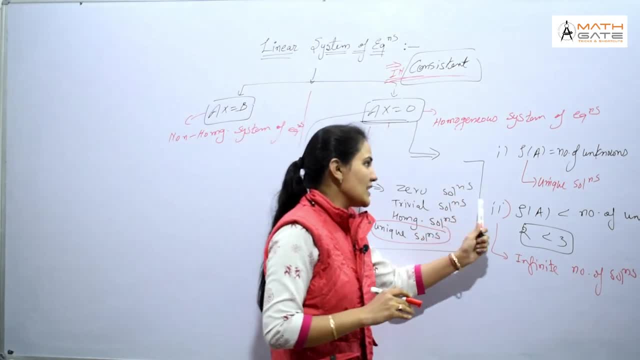 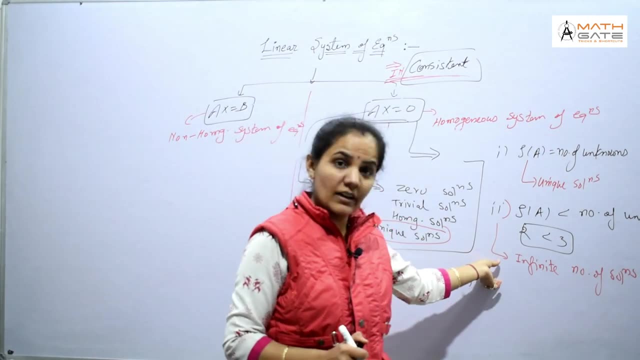 Your rank will be less. Okay, So in these two cases we discuss in homogenous system of equation. Now, students, another case comes in this. It is not a case, but it is a part of this one. What is that? 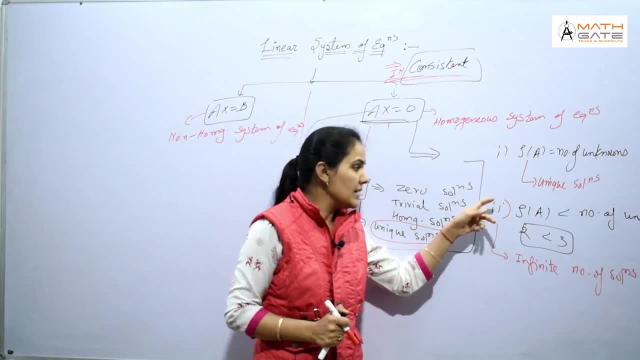 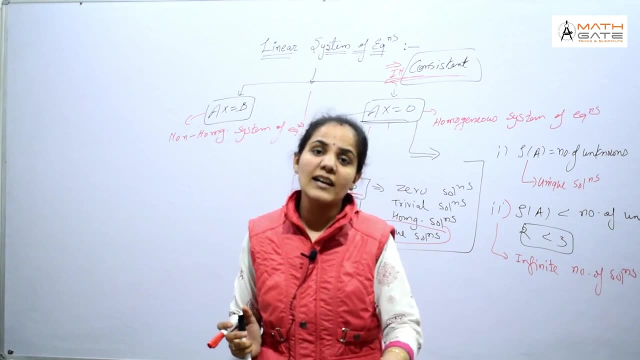 A question comes in this, that you have found out that what is there in this? The rank is less than the number of unknowns. It means the solution that is going to come is going to come more than 1.. But if you are asked, 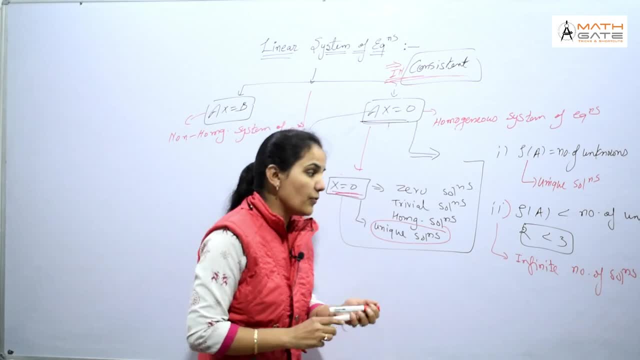 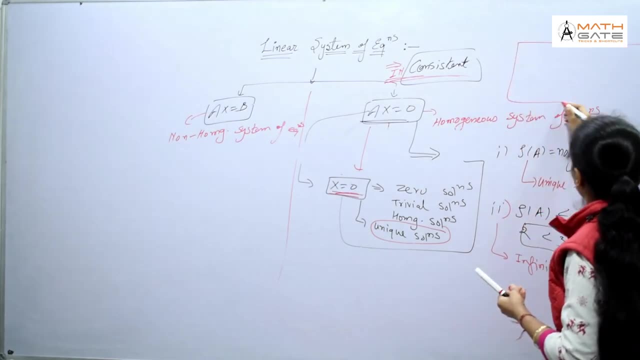 that tell me how many independent solutions are there. So you have to find out the number of independent solutions. if you have in homogenous system of equation, Then please write this property or this formula as a special note in your notebook. 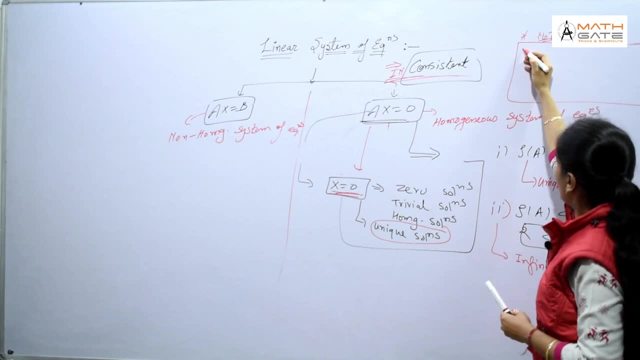 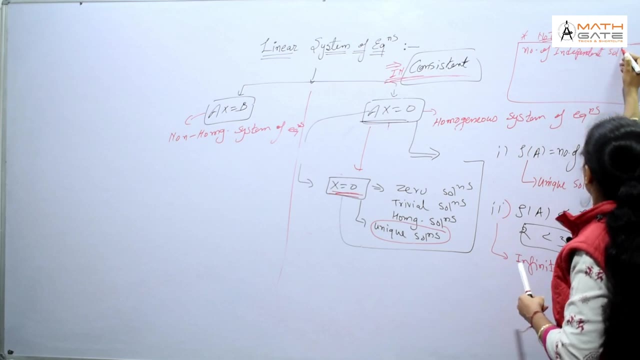 You will note it as a special note that the number of independent solutions, number of independent solutions, we denote it as P, that is equals to P. P is equals to N minus R, where N is the order of the matrix. or we can say like this: 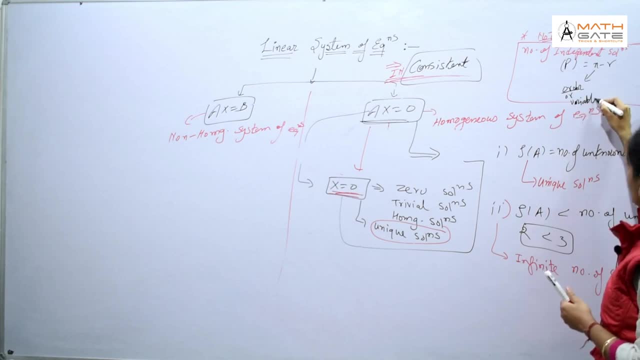 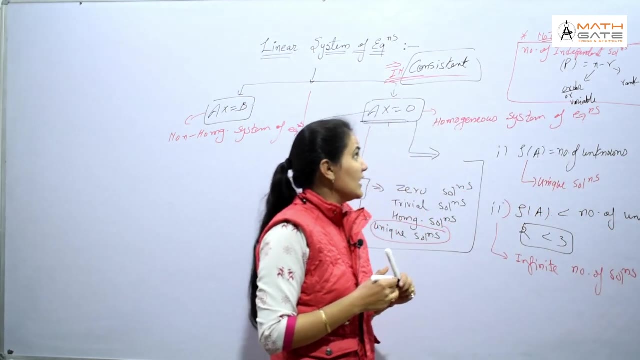 order can be done. the variable which we are talking about, that can be a variable And R is the rank of the given matrix. Let us take an example of this one. If we take an example of this one, then what is the number of independent solutions? 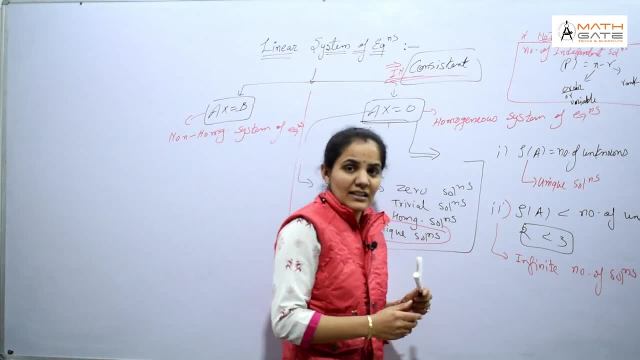 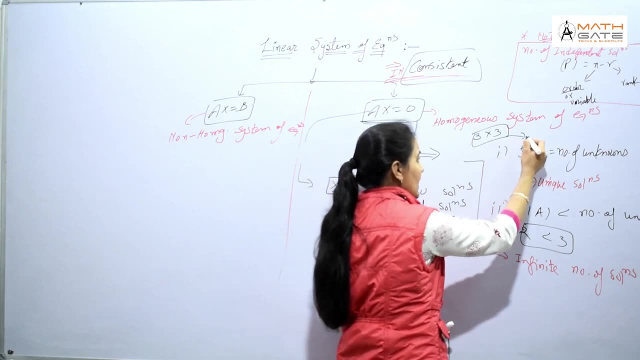 that are coming in my hand. It is P. I have to find out how many independent solutions are there. And the given system of equation suppose. what is that? The system of equation of 3 cross 3 is given, whose rank you have found out. 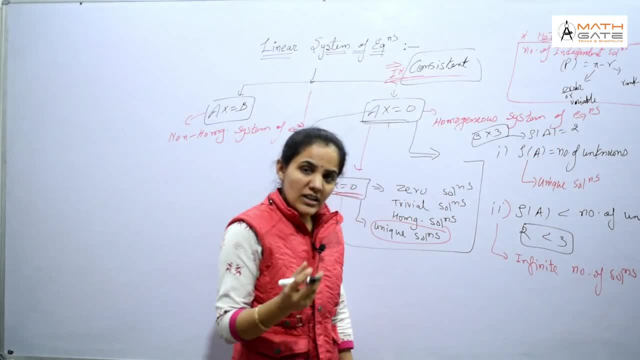 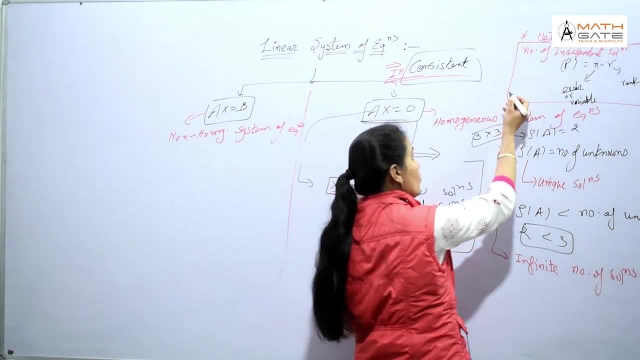 what is that? You have 2 students. Suppose you have 2 rank and the order that is coming to you is 3, or the variables that are coming to you. what is that? It is 3.. Then, if you want to find out, 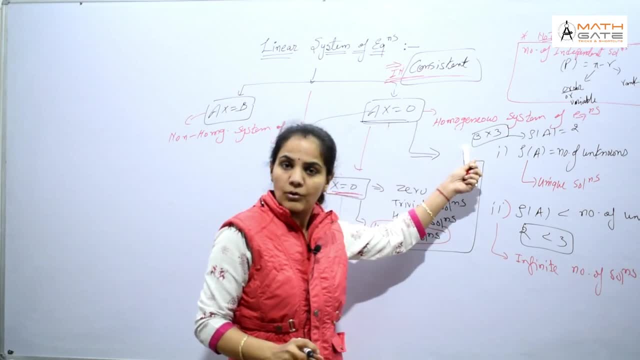 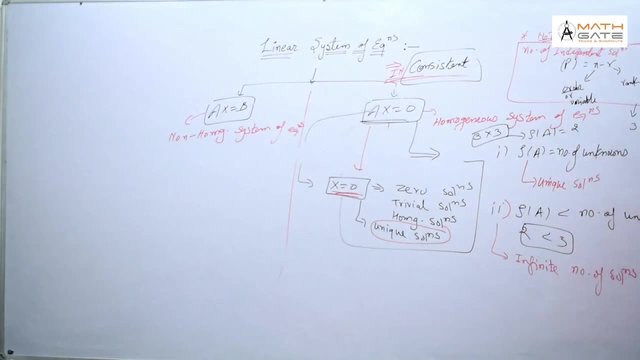 the number of independent solution for that particular system of equation. then what is the answer of that? The answer of that is going to be students. that is 3 minus 2. It means the given system of equation which we are talking about. 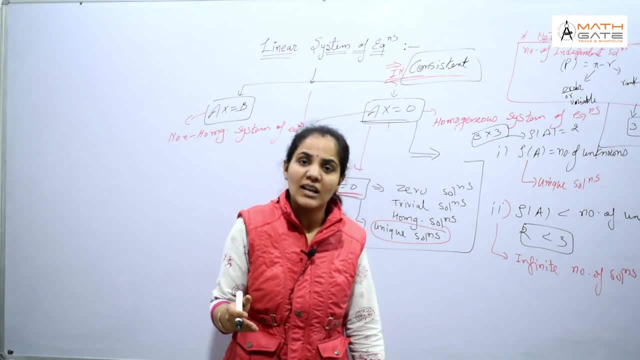 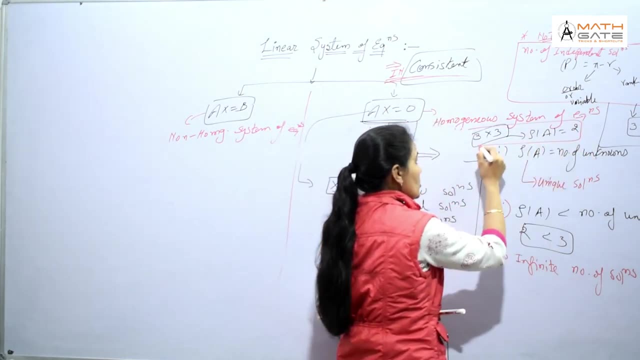 whose order we are talking about, whose order is 3, cross 3, or which has 3 variables in it- x, y, z- and whose rank is coming. 2 is coming. So, in that system of equation, what will be the number of independent solutions? 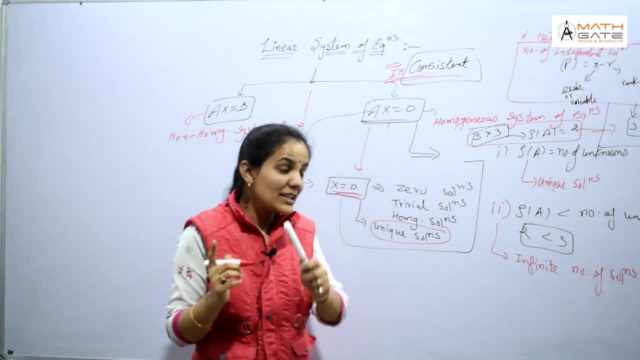 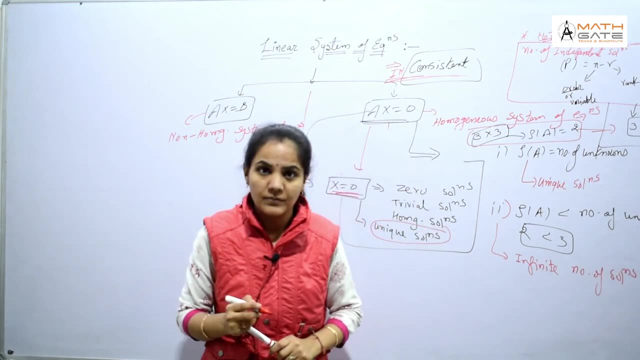 The number of independent solution will be 1.. 1 means other than this: x is equal to 0, one more independent solution will exist in that system of equation. This is called the homogeneous system of equation. The questions that come in get. 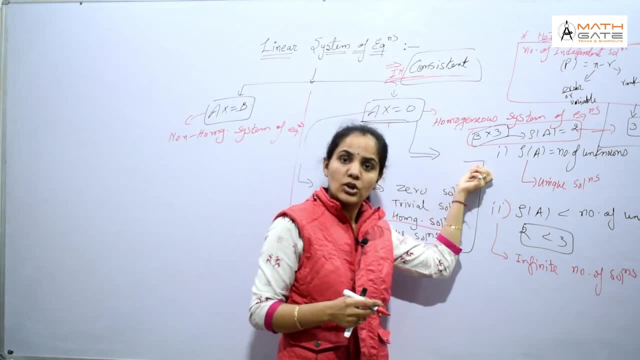 will either come to find out your rank. you have found out your rank. the number of unknowns is equal. then the unique solution is done. You have found out the rank and you have more less than 2 number of unknowns. 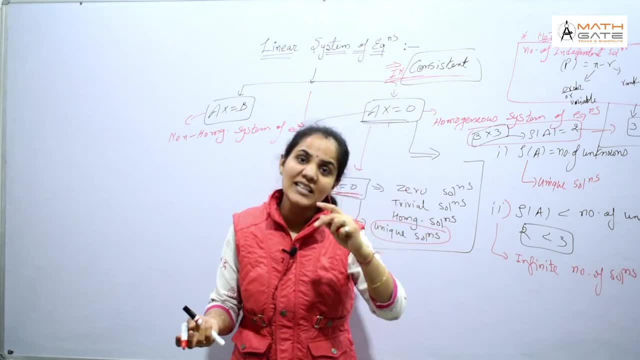 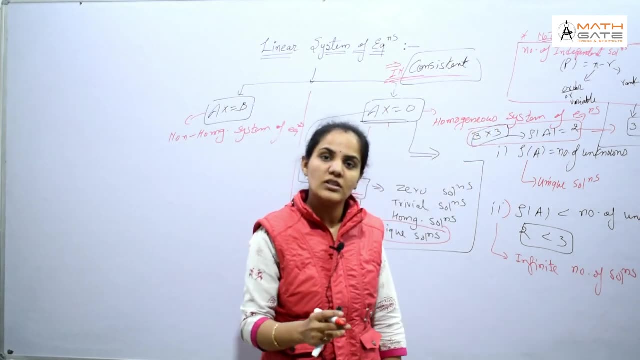 then what will happen? There will be infinite many solutions. If you want to know exactly how many solutions there are, students, then what you have to do, you have to put this formula, that is, number of independent solutions which we denote as p. 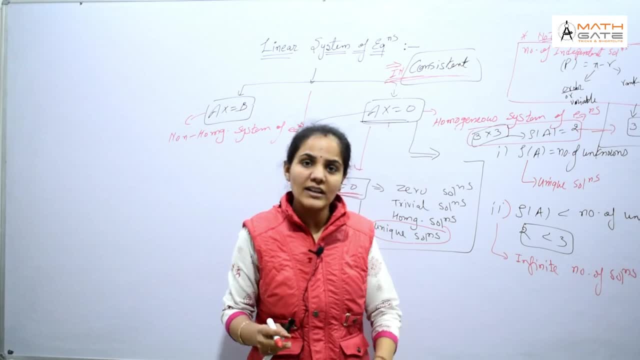 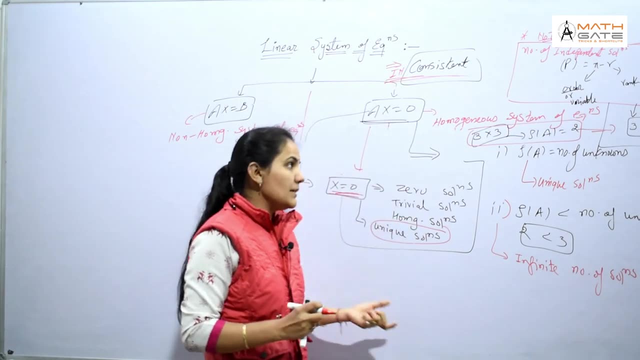 is equal to n minus r, where n is the number of variable or order or dimension which you are talking about, and r is the rank of that matrix. Getting my point? This is very important In this homogeneous system of equation. 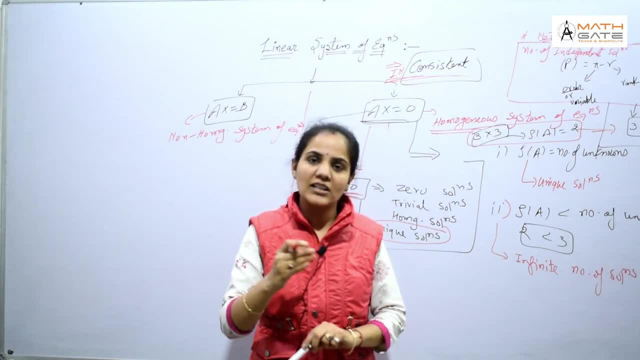 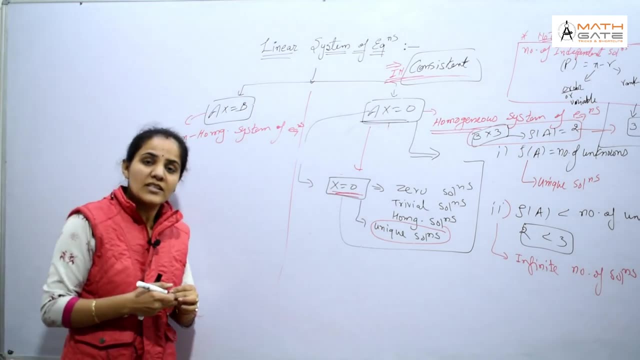 now in tools of n 19,. there is a question in EC branch and it was a very good question. we will discuss it in some time. Now come to the next part of this system of equation, that is, non-homogeneous system of equation. 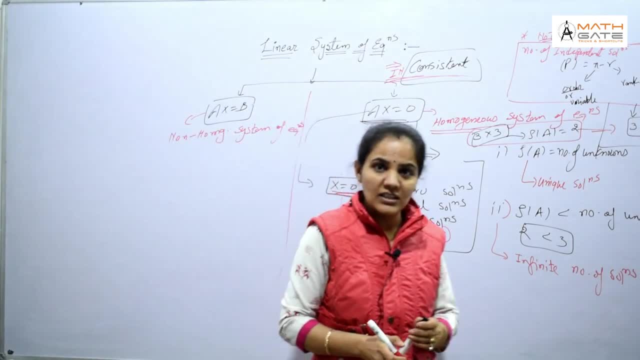 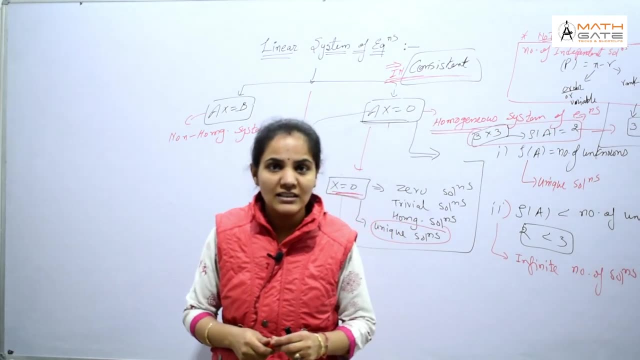 Now we will talk about non-homogeneous system of equation. So non-homogeneous system of equation which we have, students, how does it happen? In it there are equations of x is equal to b, x is equal to b. means. 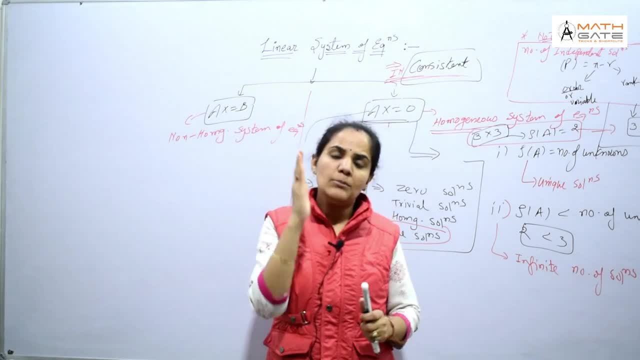 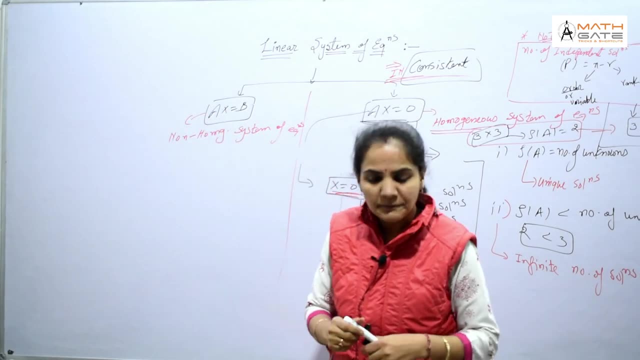 it is clear that what I have to find out here, I have to find out the rank here only if I want to know this: how many solutions can be there in this system And what solutions can be there? So there is a process to do it. 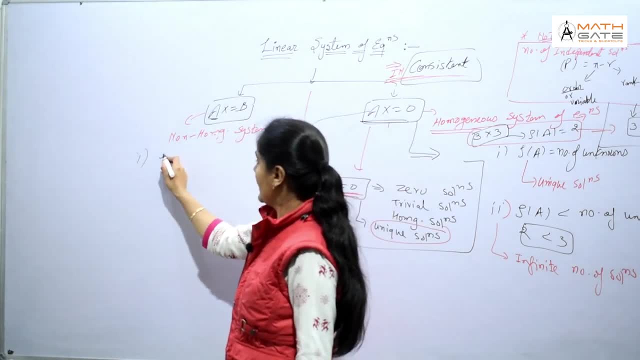 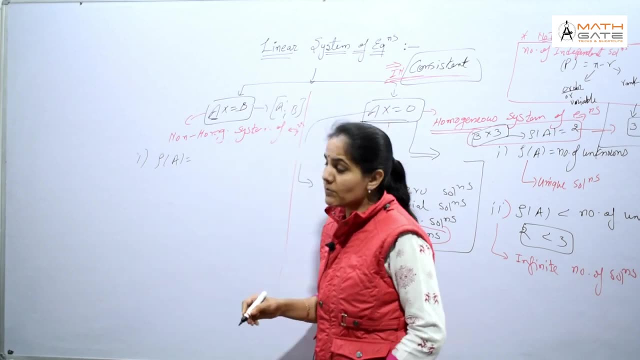 First of all, you will find out this matrix A, that matrix A's rank, And along with that, one more matrix will be made here, AB, which we call augmented matrix. This augmented matrix, we will find out the rank of AB. 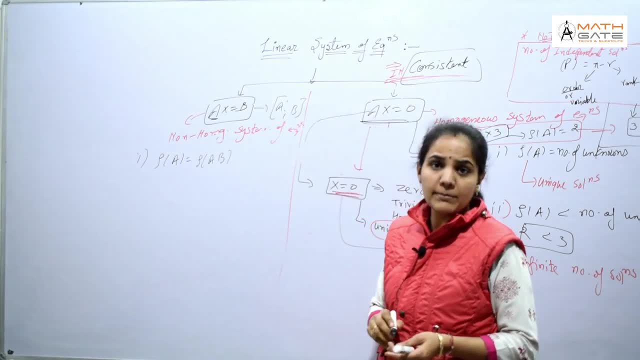 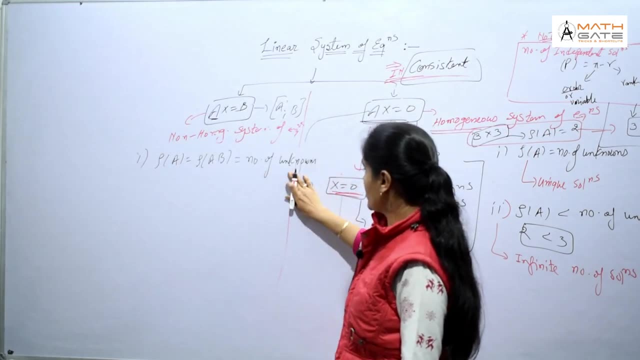 If rank of A and rank of AB, both are equal and both of them are equal to the number of unknowns. number of unknowns means you have understood here what is the number of unknowns. We will talk about the variables. 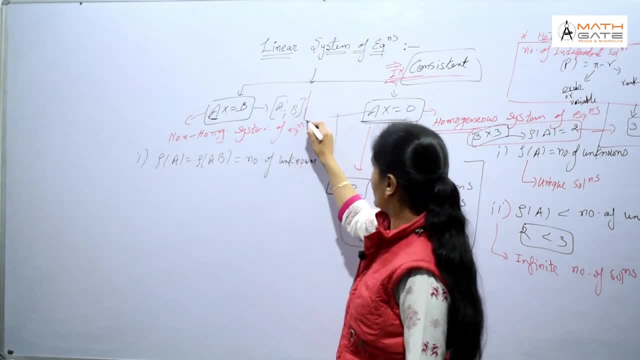 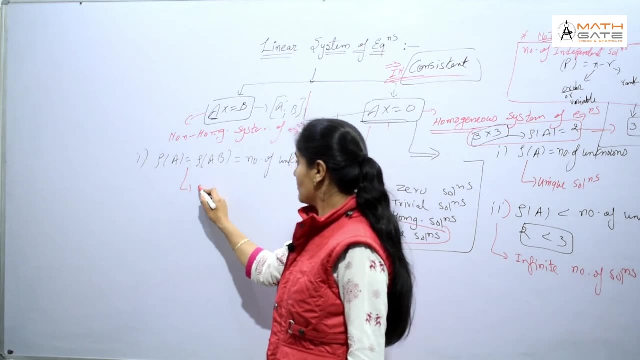 Which we are talking about, If both of them are equal to the number of unknowns, then we will say this: given system of equation which we have, students, what is it going to be? This system of equation is going to be your consistent. 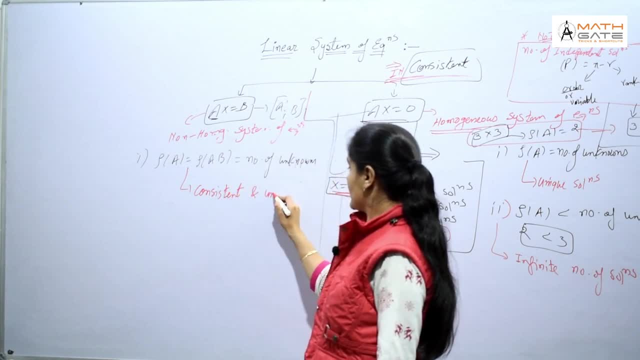 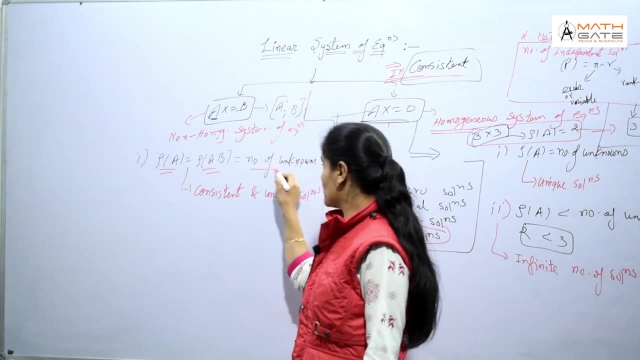 And how is the solution of this system of equation going to be? Its solution is going to be unique solution. When will it be unique? When rank of A is equal to rank of AB is equal to number of unknowns. When rank of A is equal to rank of AB. 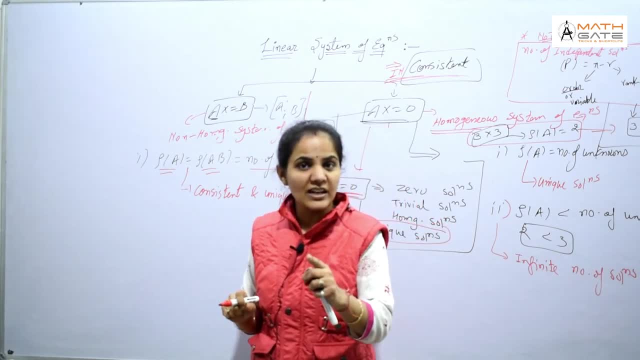 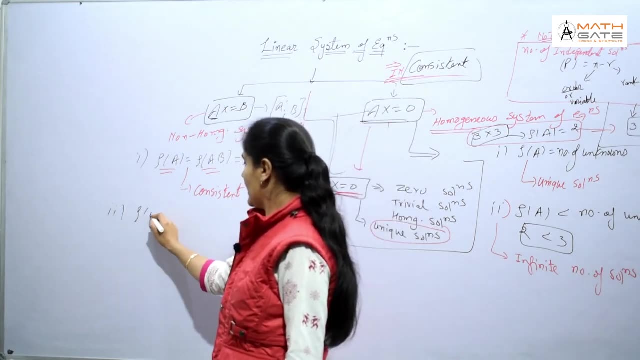 is equal to number of unknowns, Then our system will be consistent and the solution will be unique solution. The second part will come in this: if you have students, rank of A is equal to rank of AB, then you have taken it out. 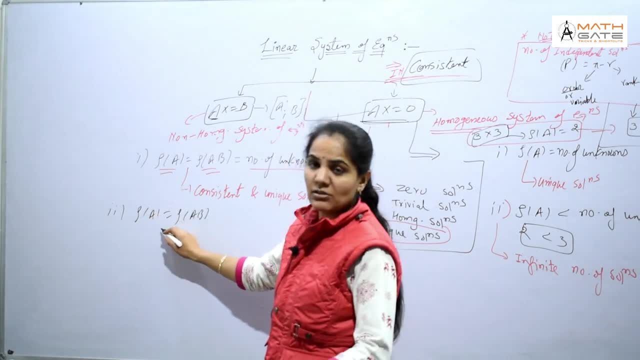 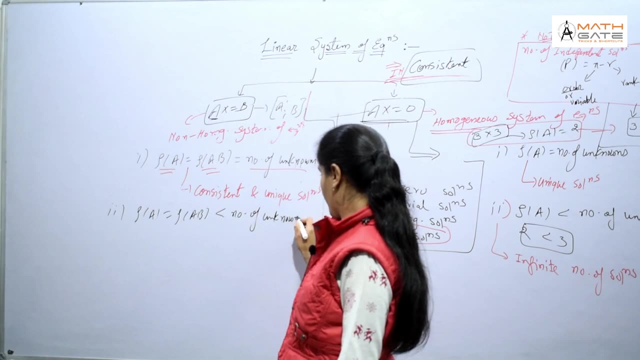 AB means augmented matrix. Ok, Rank of A is equal to rank of AB. you have found out. But what happened? This number of unknowns came less than Rank of A is equal to rank of AB, but this number of unknowns? 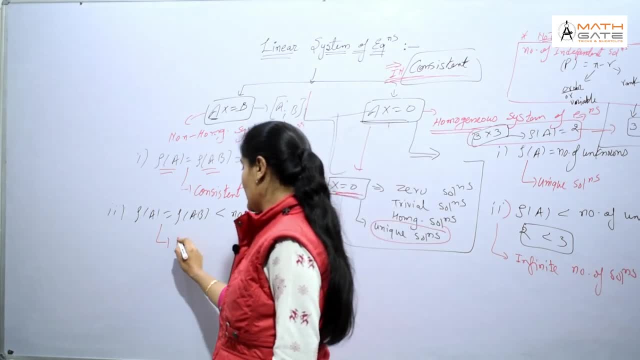 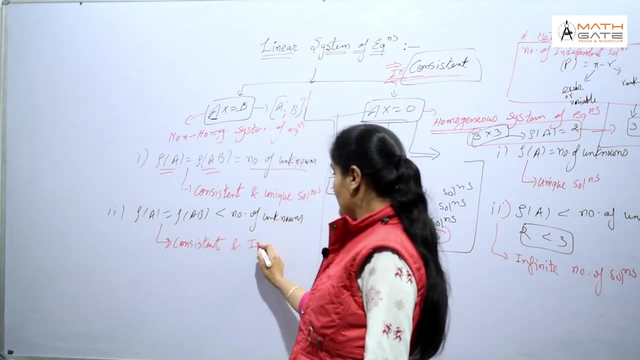 what came Less than came Then. your system will be consistent even now. The system of equations we have will be consistent even now, But what will be the solution? Infinitely many solution will be there. infinite solution will be there. 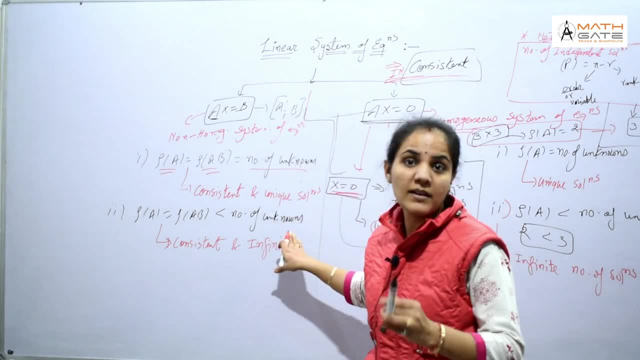 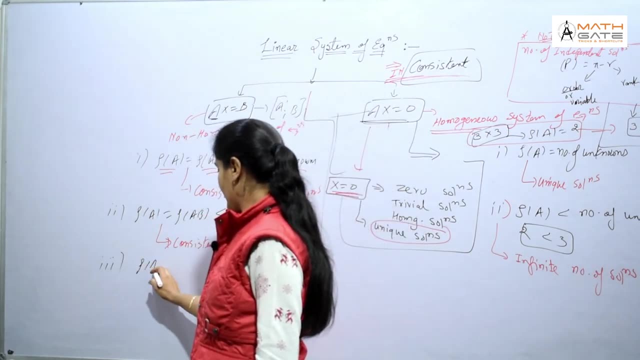 or more than one solution in this case of that system of equations will exist. Now, the last case is what If we find out that rank of this matrix is A and matrix is AB and both these ranks came? 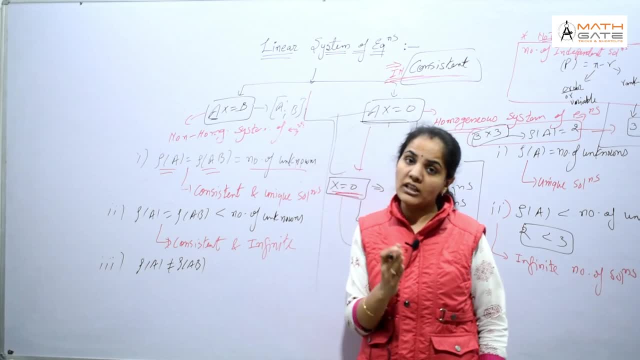 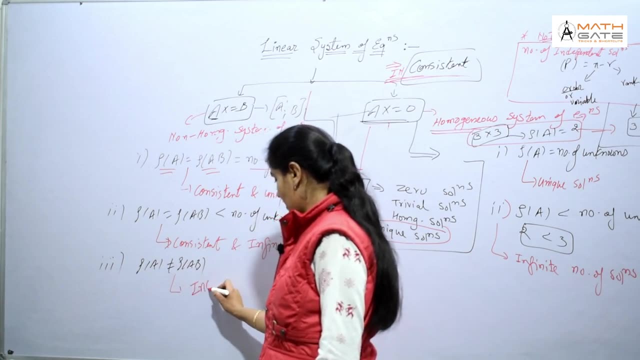 students did not come equally. If rank of A is not equal to rank of AB, then clearly we can say that the given system of equations which we have, that given system of equations, what is going to happen? It is going to be inconsistent. 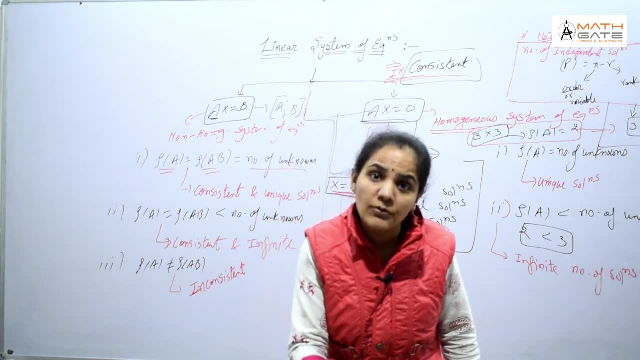 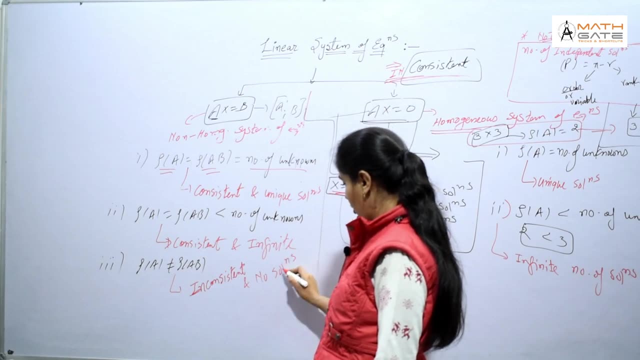 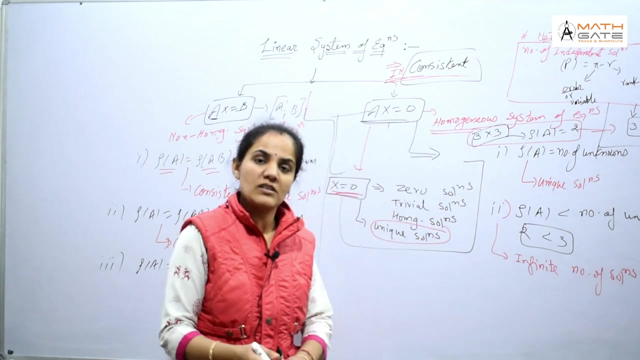 And what does inconsistent mean? That means that the solution of the system of equations is not existing. It means it will have no solution at all. No solution will exist for it. Okay, It is a very simple concept, as well as very important concept. 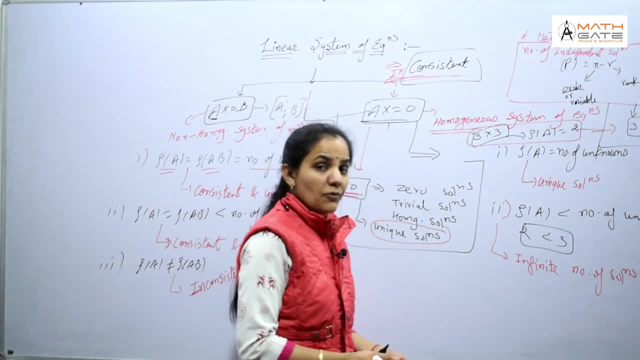 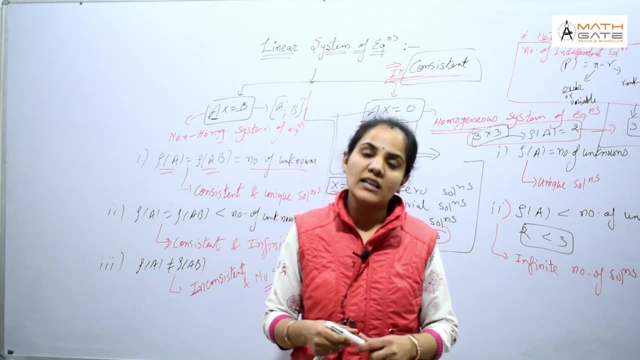 This is a good question In one gate: linear system of equations. the linear system of equations- I repeat, I will quickly revise it once- linear system of equations, what we have studied and what comes in the gate. it is of two types. 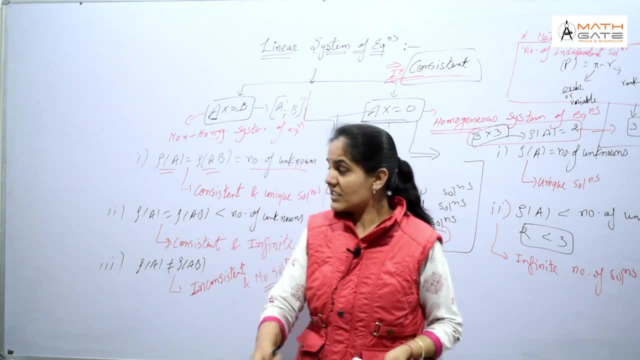 X is equal to 0, which we call homogeneous system of equations. X is equal to B, which we call non-homogeneous system of equations. X is equal to 0,. there will be two types of solutions: Means. 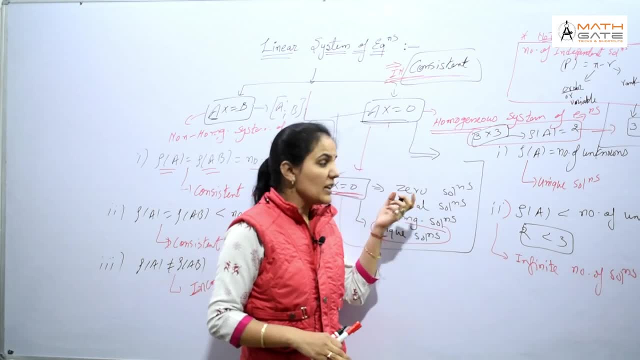 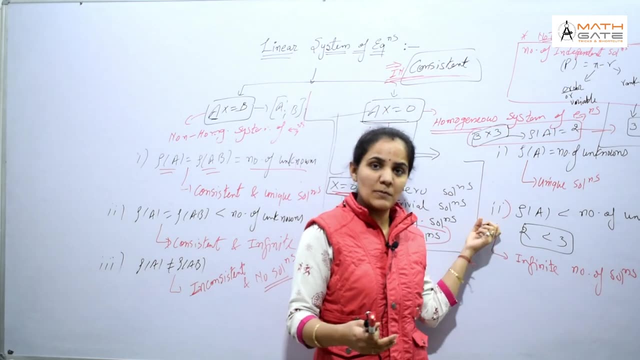 if X is equal to 0,, then its solution is always existing, Which we can call tribal solution, zero solution, unique solution or homogeneous solution. Apart from this, if there is any solution or if there is a solution in this, 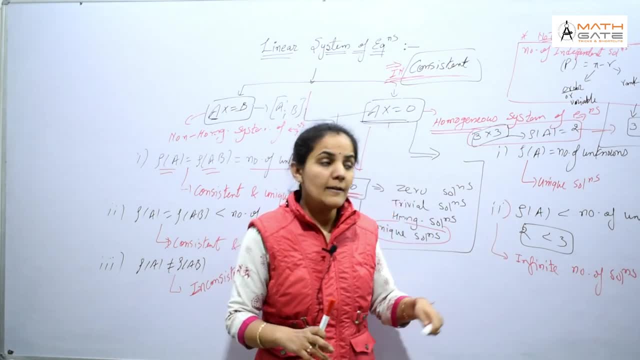 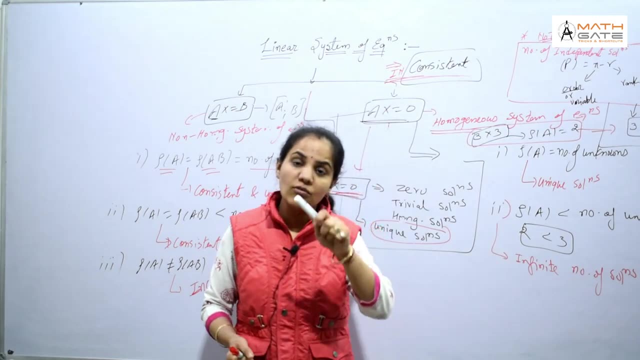 then how will you check it? You will find out the rank of A. If that number of unknowns comes once, then how will your solution be? It will be a unique solution If you find out the rank of A which is less than. 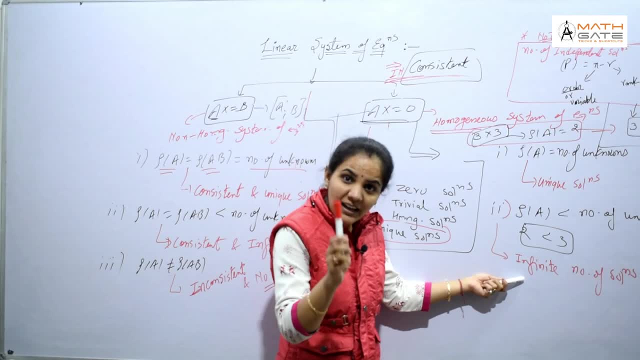 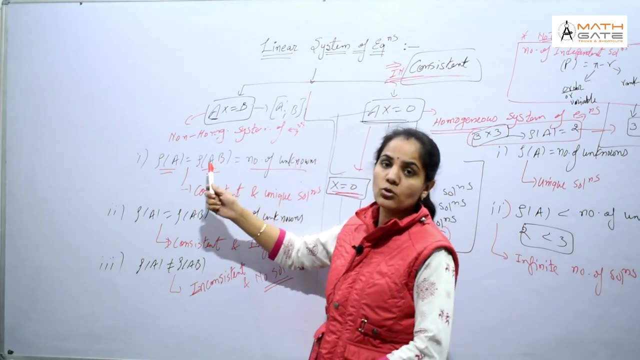 two, number of unknowns or students, then how will your solution be? Infinite number of solution Getting my point. Now come to the next one. If we come to this, then AX is equal to B, which we are saying: 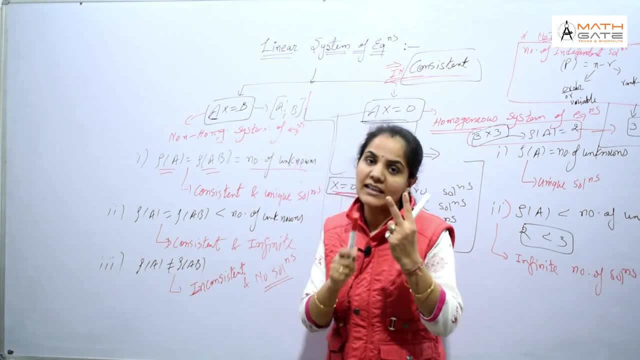 non-homogeneous system of equations. This AX is equal to B. you have to remove two colors. you have to remove matrix A also and matrix. you have to remove matrix AB also. This matrix AB we call augmented matrix AB also. 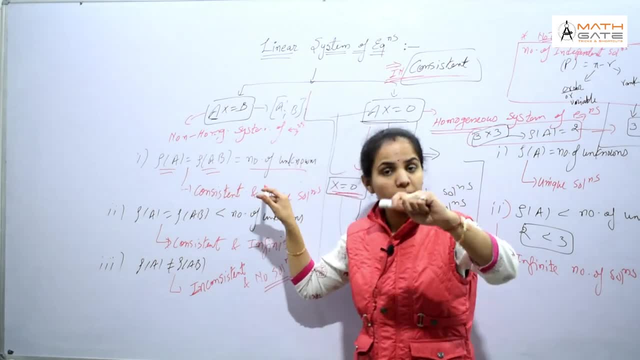 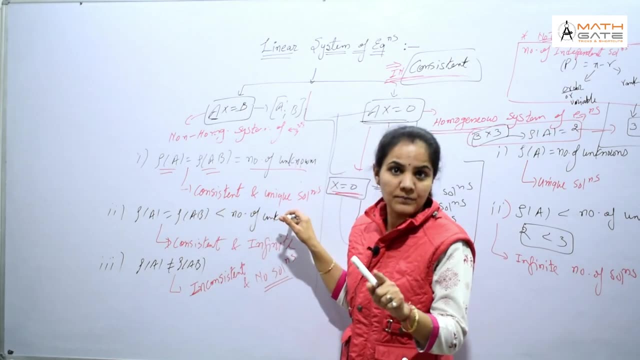 So rank of A is equal to rank of AB is equal to number of unknowns. if it comes, then we will say: what is this? Our system is consistent, and what is it? It is a unique solution for this system. 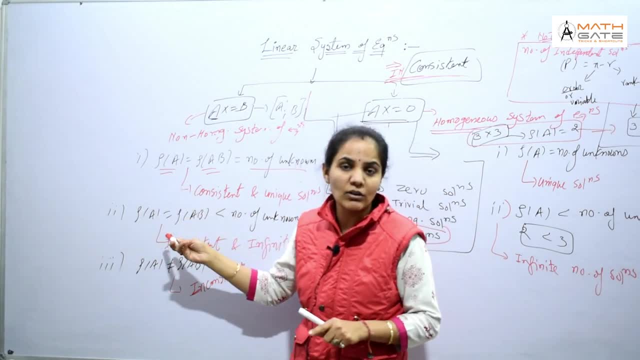 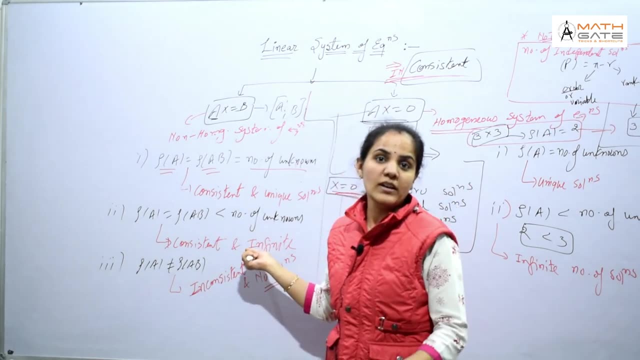 If rank of A and rank of AB is equal, but that number of unknowns is less than then, my system will remain consistent. but how will the solution of the system be? There will be infinite solutions or infinitely many solutions. 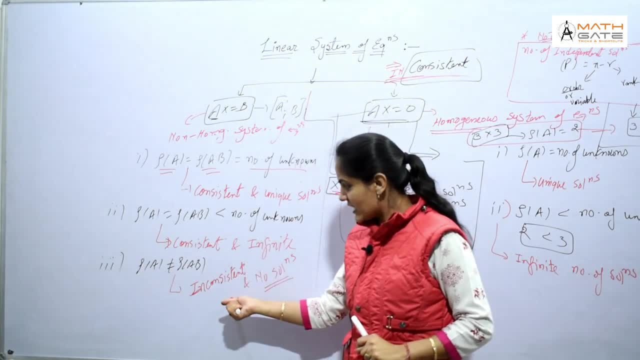 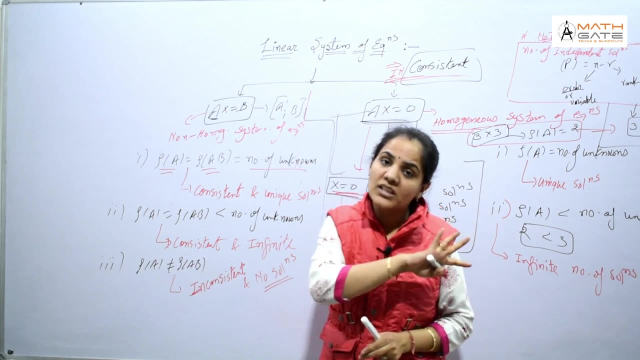 or there will be more than one solution. And in the last case, is what? If rank of A is not equal to rank of AB, then our system is said to be inconsistent means there will be no solution of this. and having no solution 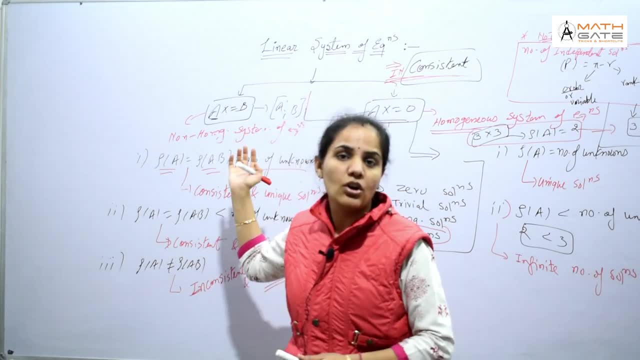 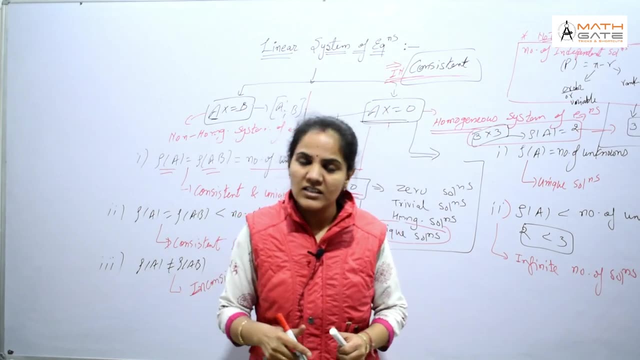 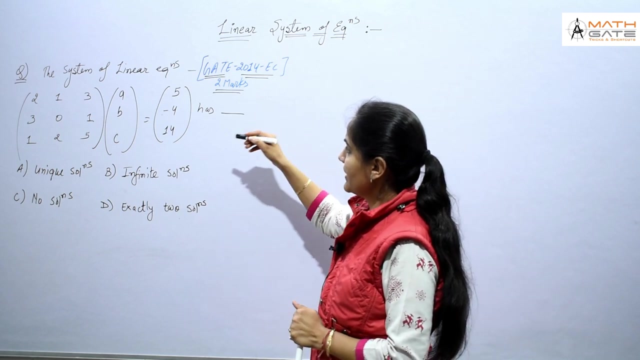 Okay, now let us discuss question based on these system of equations, or homogeneous or non-homogeneous? what kind of question has come in both in GET? let us discuss. The question is the system of linear equations. 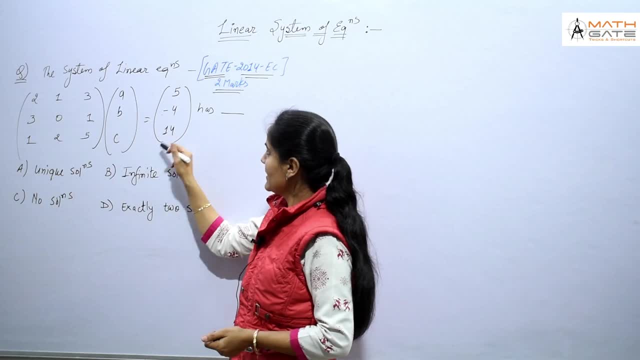 2, 1,, 3, 3, 0, 1, 1, 2, 5,. ABC is equal to 5 minus 4,. 14 has options are. unique solution, infinite solution. 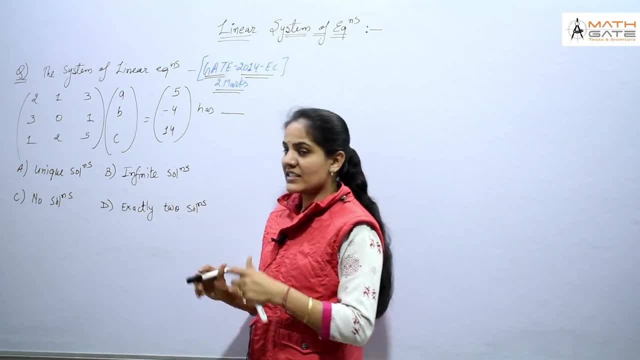 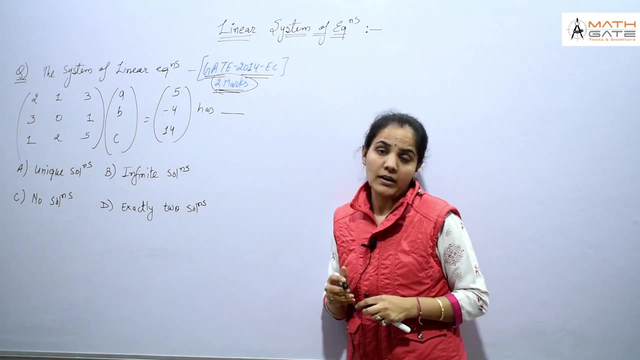 no solution, or exactly 2 solutions. This question came in GET 2014, EC branch of 2 marks weightage. Okay, now let us discuss the question. first of all, you can understand. 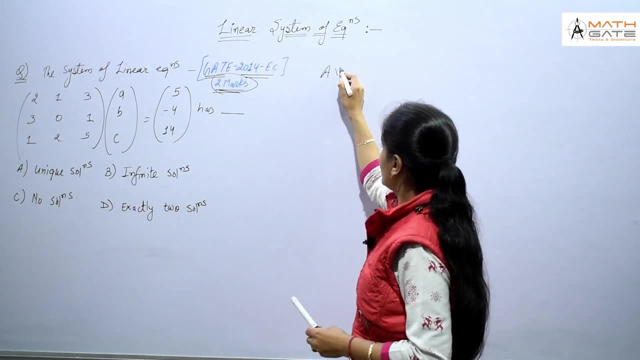 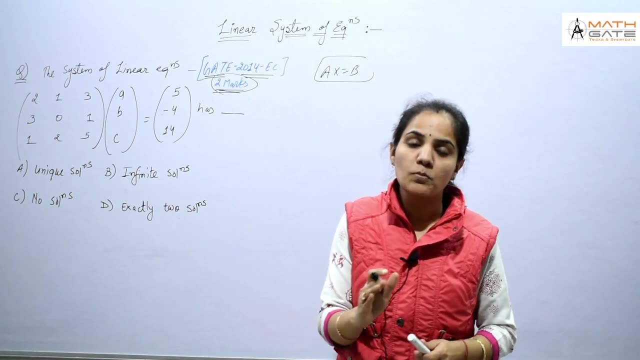 by looking at this question, that this question is: AX is equal to B concept. it is not of homogeneous system of equations. this is not of homogeneous. this is: AX is equal to B type of solution. okay. 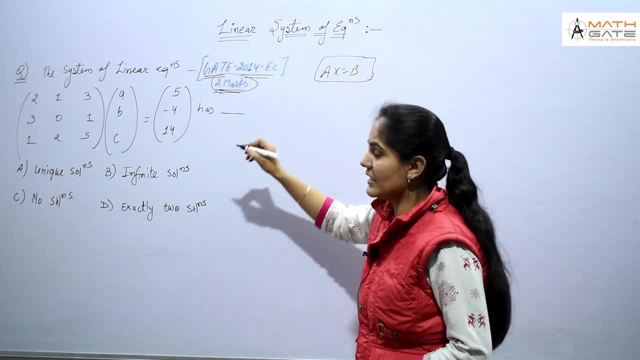 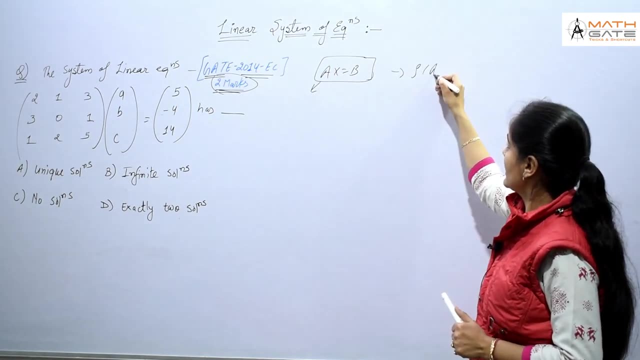 type of question is: AX is equal to B. type of: if this is the question, what we have to do, students, I have to do here- I have to find out the rank of matrix A. just now we have discussed. 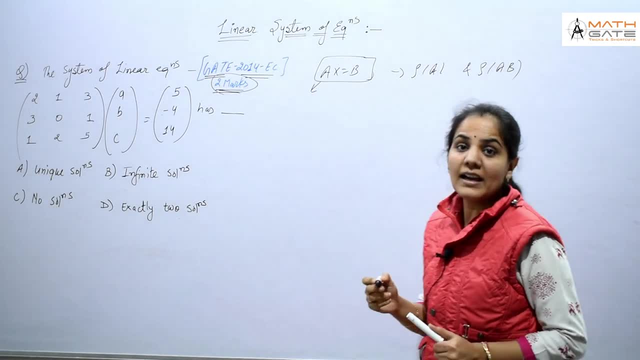 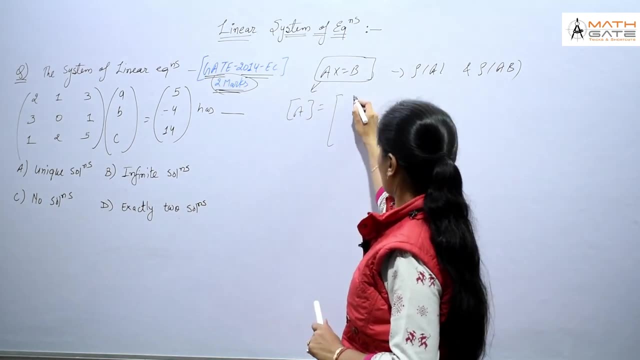 matrix A and matrix AB. AB is our augmented matrix. we have to find out the rank of these two. so first of all, if you make matrix A, then matrix A will be 2, 1,. 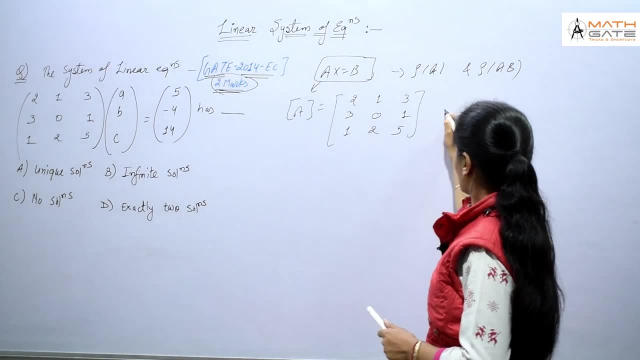 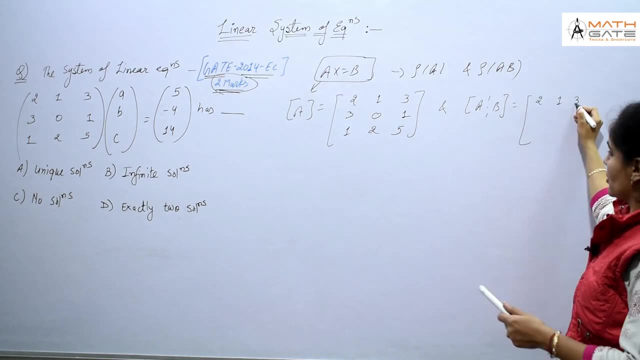 3, that is 3,, 0,, 1, and it is 1,, 2, and 5, and if you make matrix AB or augmented matrix AB, then that will be 2, 1,. 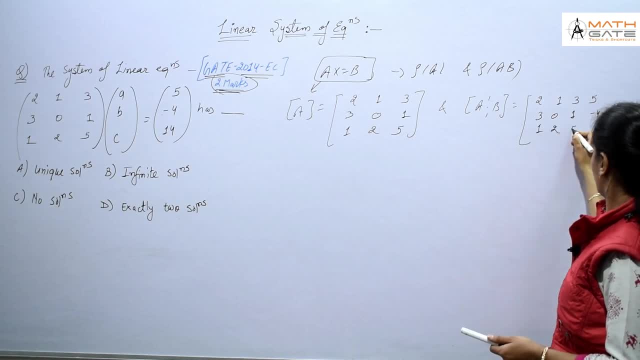 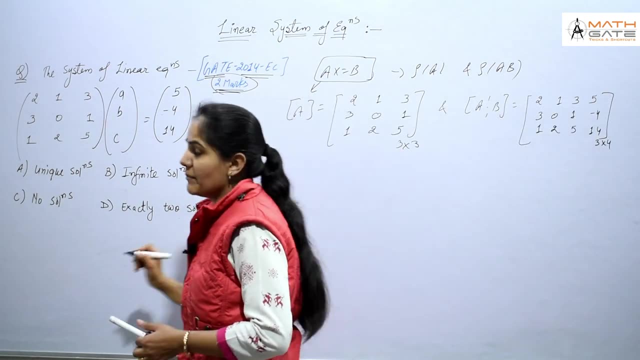 3, and here 5,, that is 3, 0, 1, minus 4, and this will be 1, 2, 5, and this will be 2, 3, 0,. 1, 1, 0, 0, 1, 1, 1, 0, 0, 1, 0, 1, 1, 1, 1, 1, 0,. 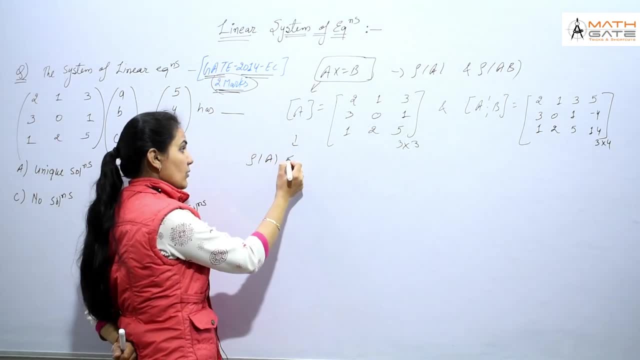 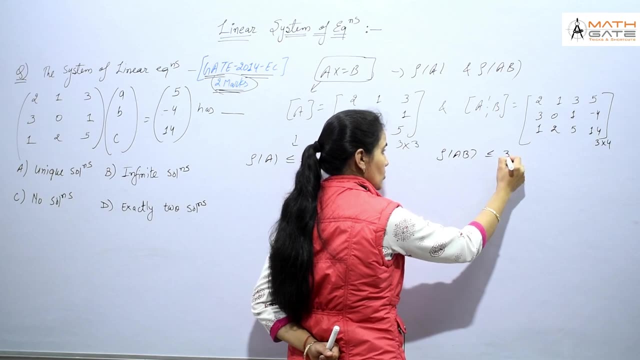 0, 0, 0, 0, 0, 1, 1,. If we talk about AB, then rank of AB will also be the same: less than or equal to 3.. Because rank of A is less than or equal to minimum of MN. 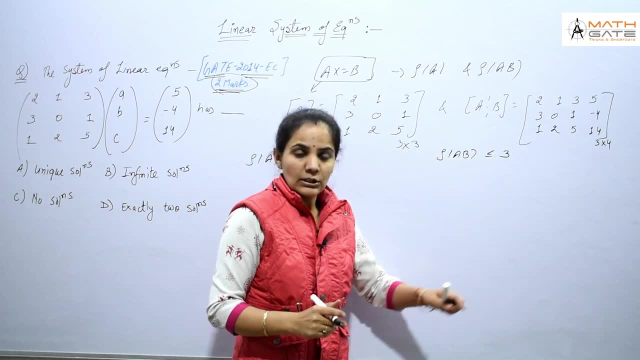 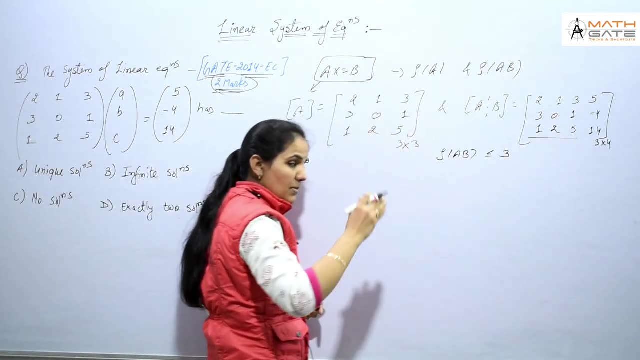 Here, minimum 3 will be there. Here, minimum 3 will be there. So what you have to do, students, if you solve matrix AB, if you solve this matrix AB, then this matrix AB will also give you the rank of A matrix and AB matrix. 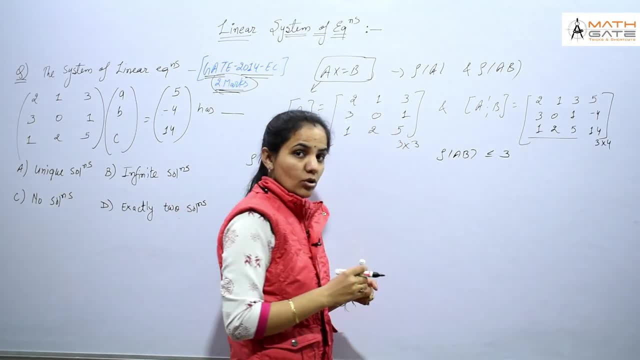 That means if you solve this matrix AB in the first 3 columns, then these first 3 columns are giving you the rank of matrix A. They are also giving you the rank of A matrix. Along with that, they will also give you the rank of matrix AB. 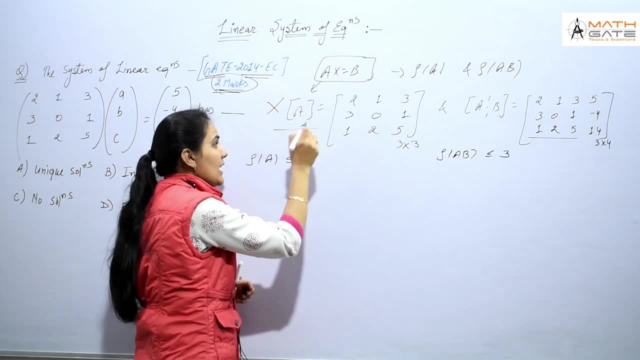 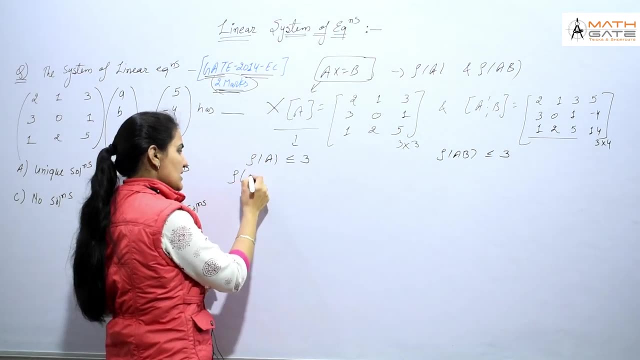 So what you have to do is you don't have to go to this concept, You don't have to solve matrix A separately. Now what we will do is we will start directly from rank of matrix AB, And rank of matrix AB is also less than or equal to 3.. 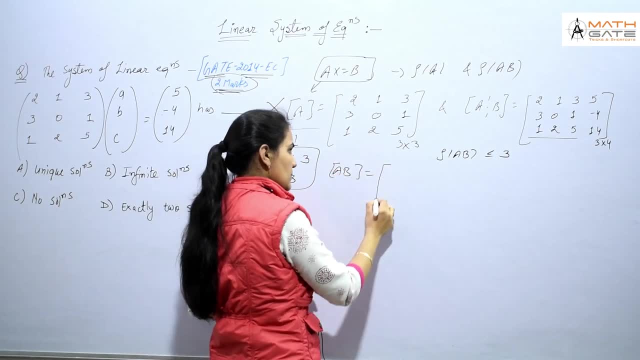 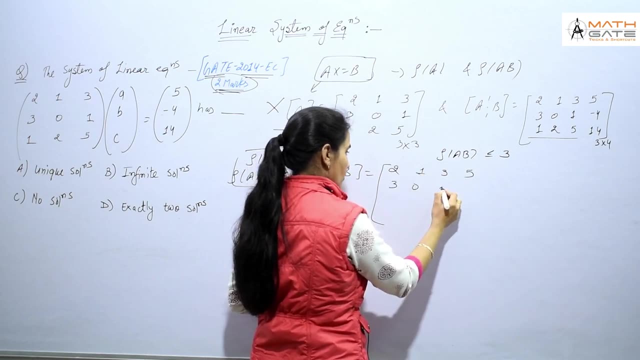 So we will take matrix AB first, which you also call augmented matrix. Take this: 2, 1,, 3 and 5.. It is 3, 0,, 1.. 1 and minus 4, it is 1,, 2,, 5 and 14.. 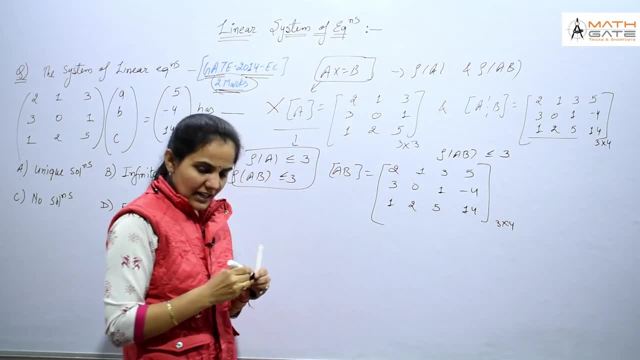 The order of this matrix is 3 cross- 4.. See, first of all, what you have to do is if you have to solve any matrix or if you have to find the determinant of any matrix. why do you have to find it? Because you have to find the rank. 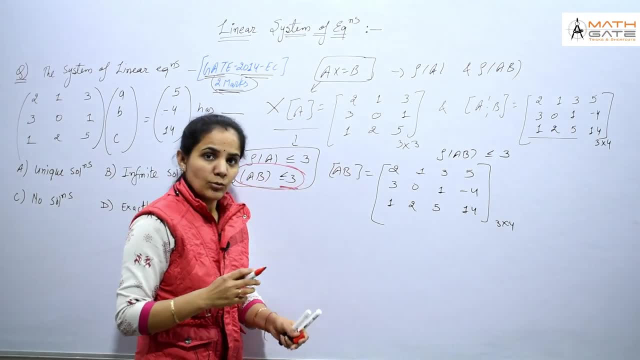 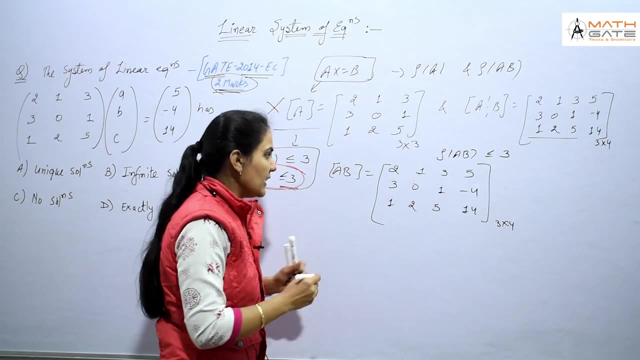 If I know this matrix, for matrix AB is less than or equal to 3, its rank, then it means that for this I have to find the determinant of all the miners of 3 cross 3.. So, before going to the determinant concept, what you have to do is 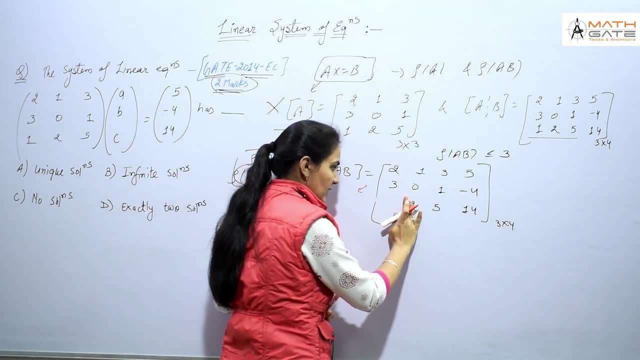 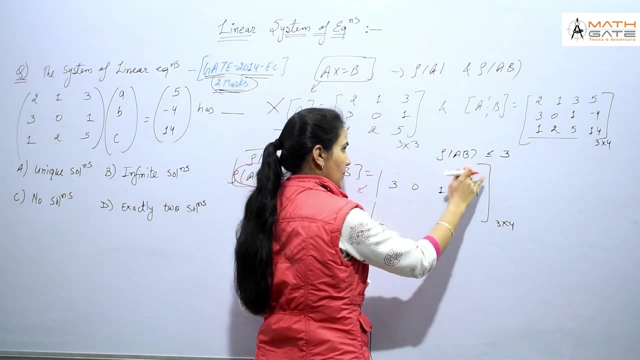 make this question a little easy, Write this question like this: This first and last row. we will interchange R1, interchange R3.. We will write this last row on the upper side And we will write the upper one on the lower side. 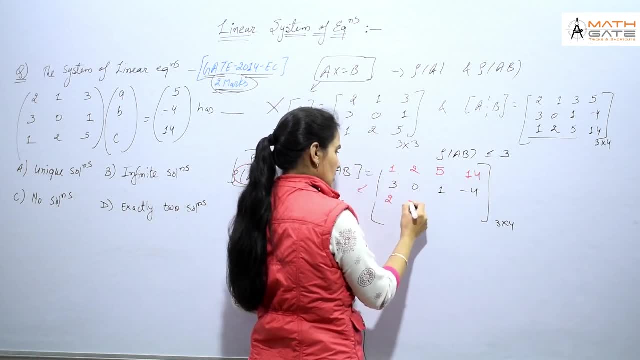 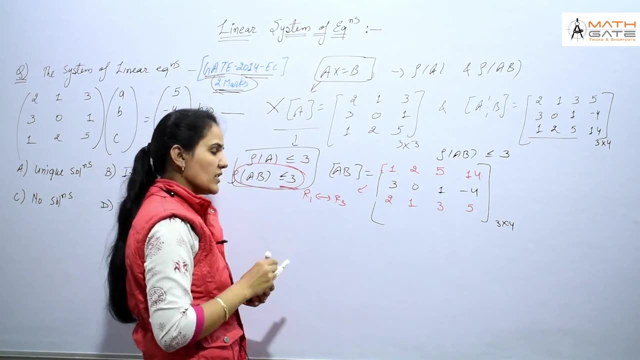 So 1,, 2,, 5 and 14.. And this will be 2,, 1,, 3 and 5.. The rest will remain as it is. Now, what is going to happen Now? you have to apply a simple transformation. 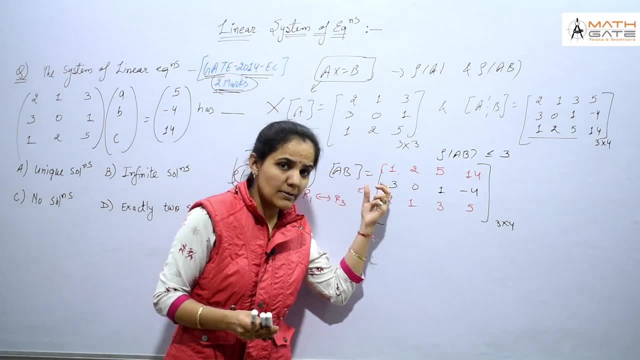 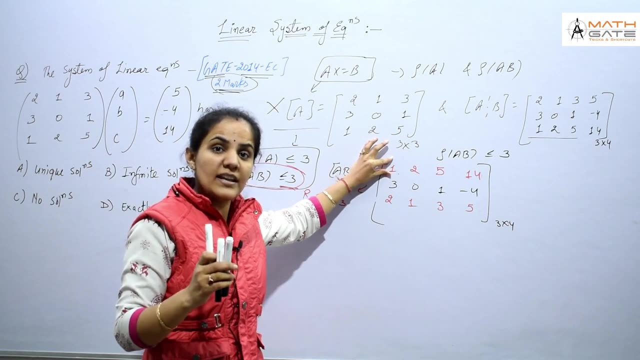 The basic rule of elementary transformation is that if you have to apply a transformation on any row, you have to see in that if the first element of that matrix is 1, then try to make elements below 1 also 0. What will you do? 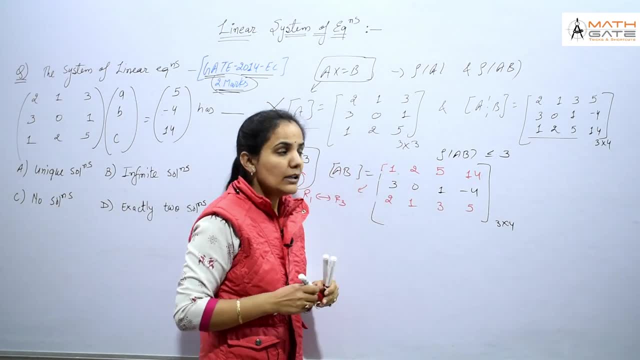 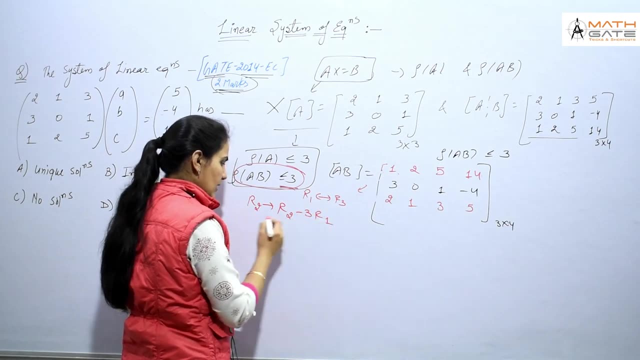 You will try to make elements below 1: 0.. So, first of all, we can apply this transformation on the top. We will do it in the place of R2.. Students: if R2 minus 3, R1.. And same we will do it in the place of R3.. 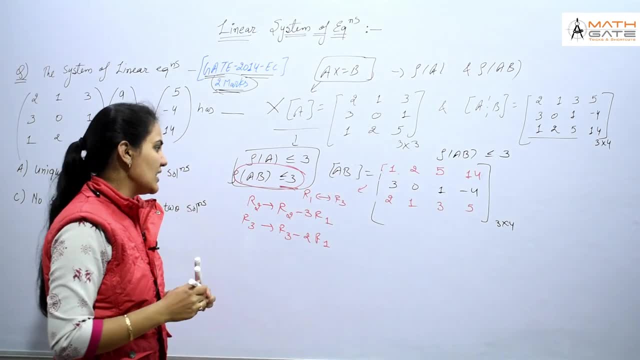 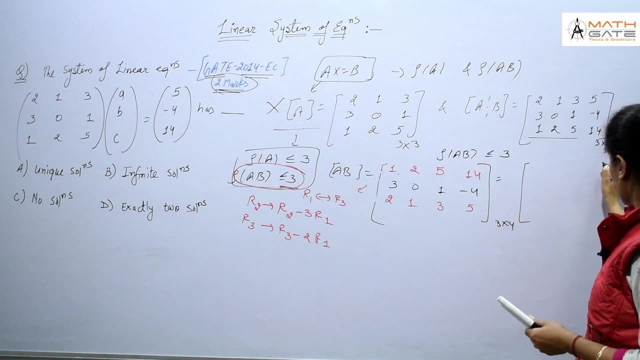 What will R3 do? 2 R1.. So this matrix of mine will change After applying some transformation in it. the value will change. What will happen? We will discuss that here. If I apply this transformation in it, then my matrix will be made. 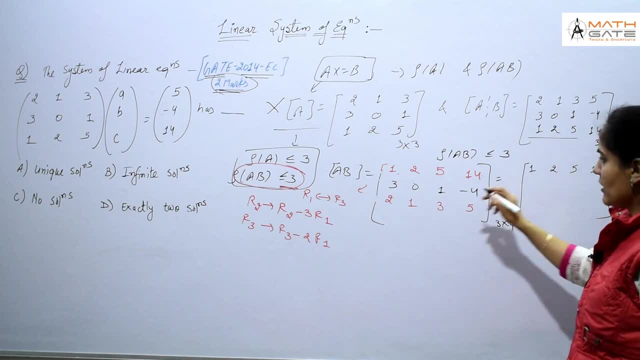 This will remain as it is: 1,, 2,, 5 and 14.. This became R3.. At the place of R2, R2 minus 3. R1 means 3 minus 3: 0.. This will become 0 minus 6 minus 6.. 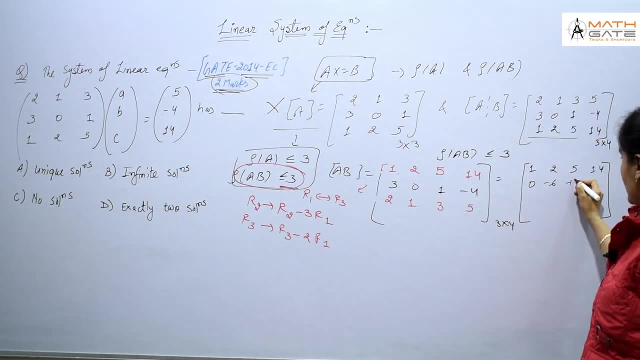 This will become: how much do you have? 1 minus 15, that is minus 14.. Sorry, 1 minus 15 minus 14 and minus 4.. And if you solve this, then you will get minus 46.. In the same way, if you apply it in the place of R3,. 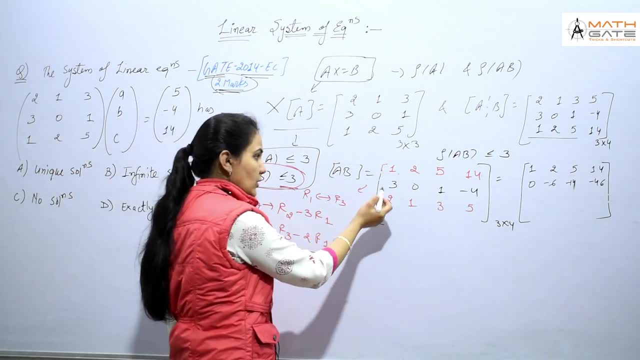 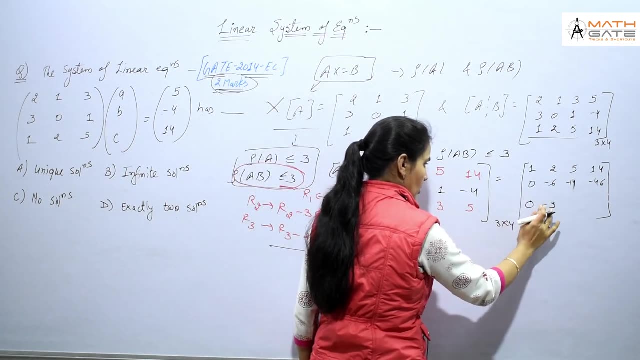 R3 minus 2 R1.. So this will become 2 minus 2: 0.. This will become 1 minus how much? will it be? 4 minus 3.. And this will become next element. you have 3 minus 10.. 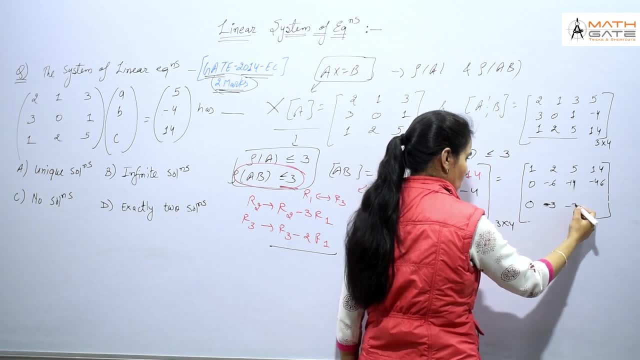 That is equal to how much will it be? 3 minus 10.. If you did, then how much will it be Minus 7.. And this will become 5 minus you will do 28. Then you will get what. 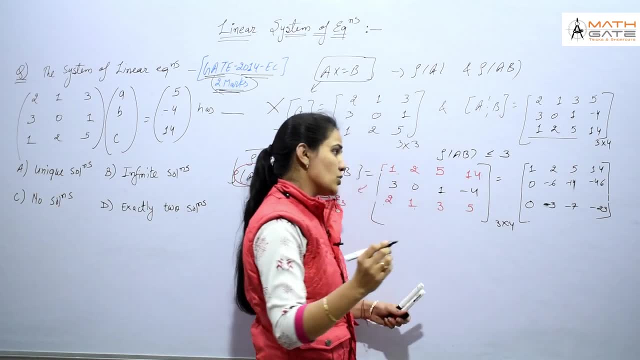 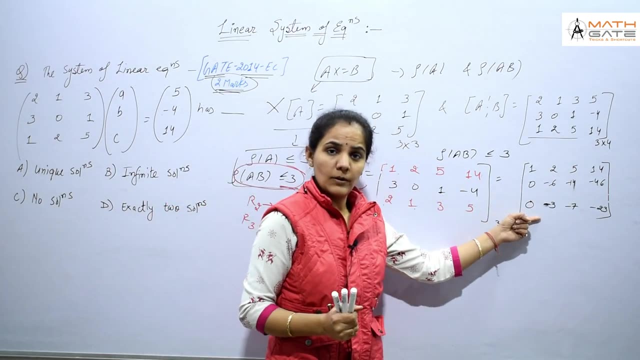 Minus 23.. Now, if any student, if any student has discussed our last video, which is the rank of matrix, or have seen it properly, then that student from this given matrix can also tell the rank of this matrix. 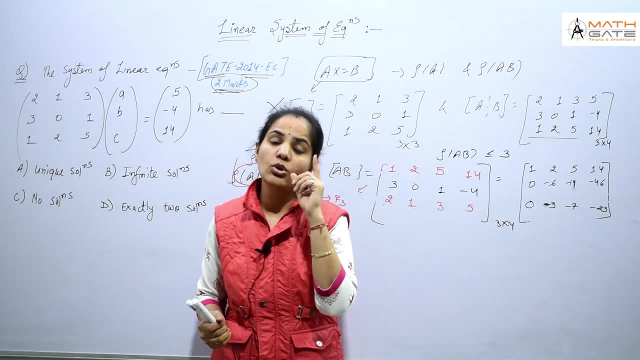 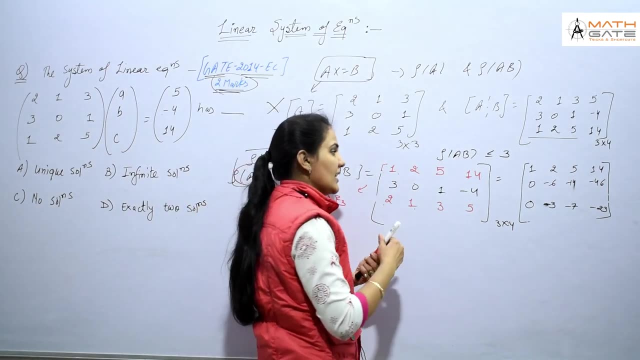 Along with that, from this given matrix, you can see what you can get out of it. you can also get out the determinant within a fraction of second. Why? Because as soon as you see this matrix, properly observe that, you can clearly see. 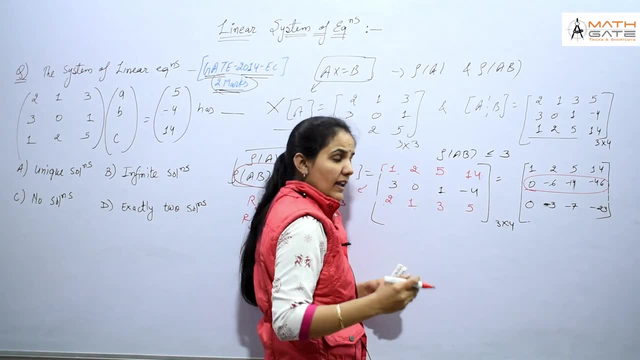 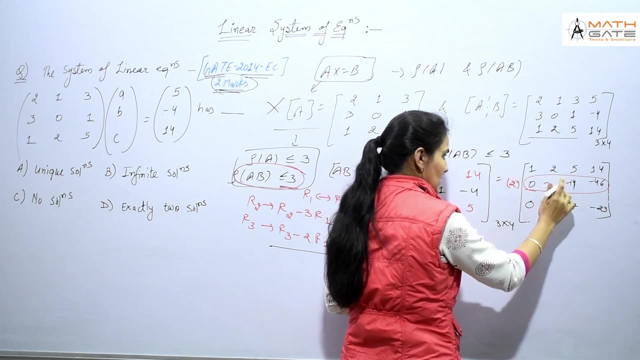 that this matrix, which I can see from its second row, if I get out from its second row, if from its second row I get out 2 common from its second row, then these elements will become what? 3. This element will become: 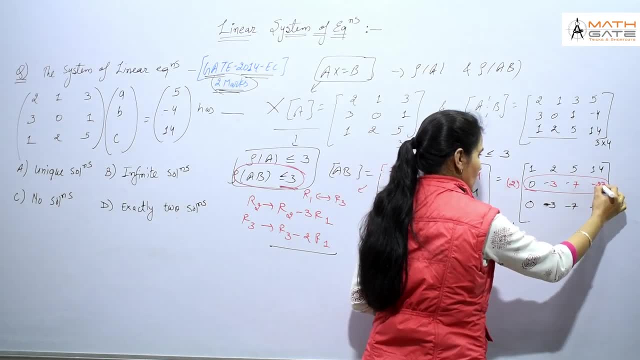 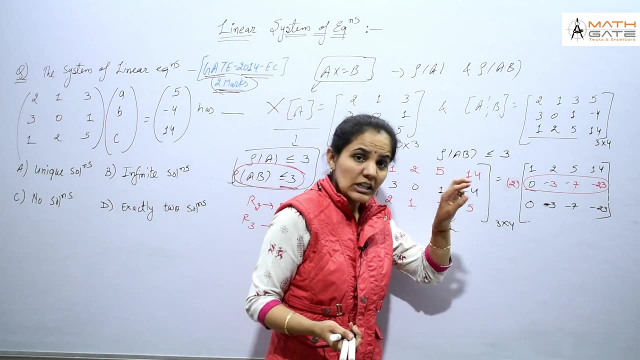 how much 7.. And this element will become how much Minus 23.. Now, as soon as you see this, you can say that in the very first video we had discussed that. if in any two rows 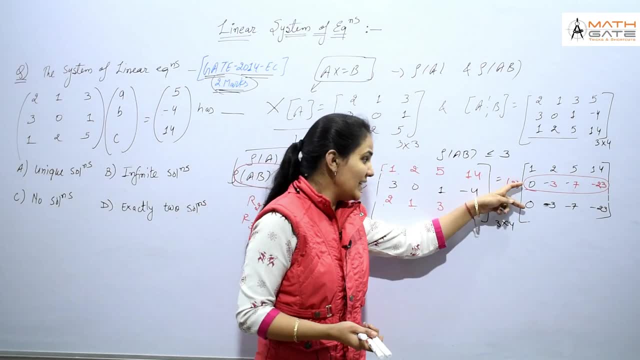 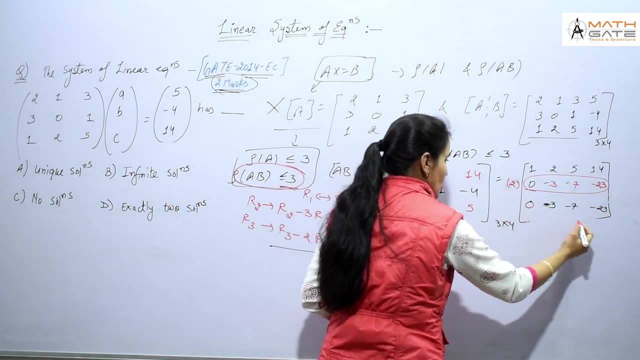 or if in any matrix two rows or columns are identical, then the determinant of that matrix is equal to always 0.. So what will always happen? It will always be 0.. This means this matrix which I have taken. 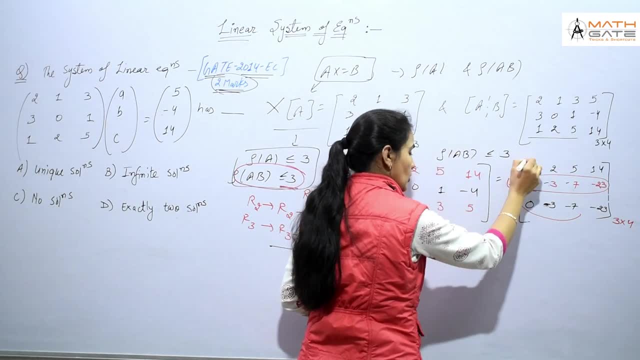 what is that matrix? It is of 3 cross 4.. In this 3 cross 4 matrix, whether I take this minor of 3 cross 3, whether I take this minor, whether I take any minor in this 3 cross 4 matrix. 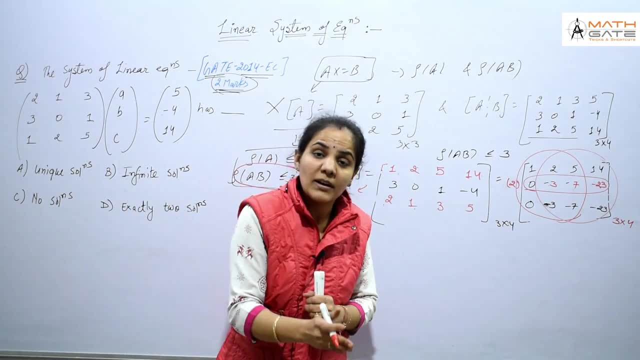 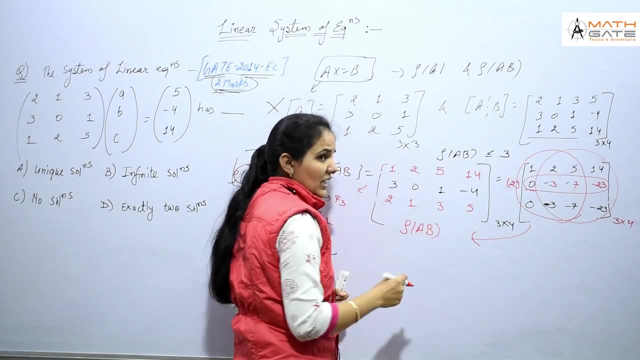 no matter how many minors you take in, 3 cross 3, what is the determinant of all of them? It is going to be 0.. It means what happened, students, That it was clearly shown to you that the augmented matrix, which is AB. 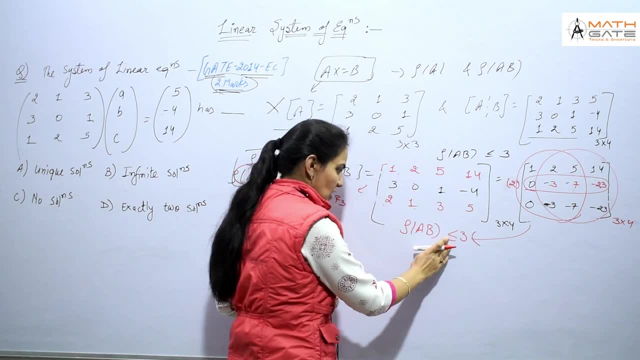 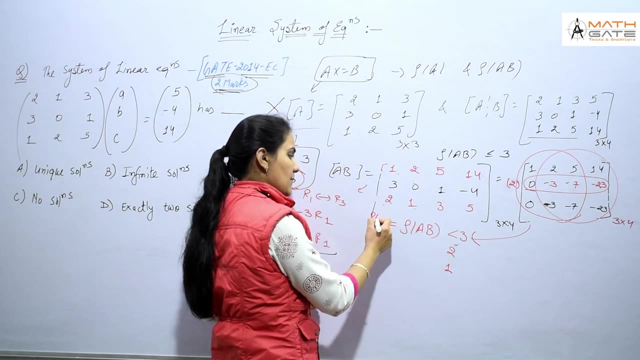 what will be its rank? It will be less than 3.. It cannot be equal Now. less than 3 means you have options: either it will be 2 or it will be 1.. Same with the rank of AB. 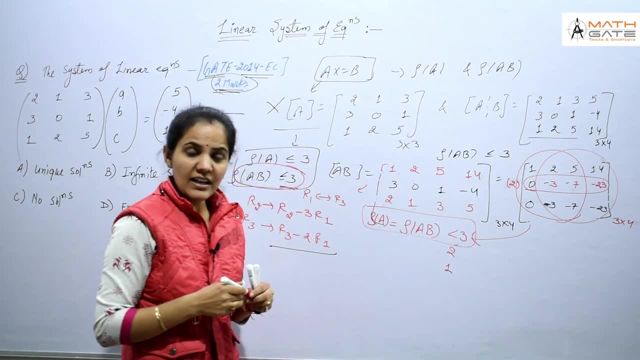 For both A and AB. this is going to be the case. Now you have come to know that. what is the rank of A and AB? It is less than 3.. Now, in less than 3, it is 2 or it is 1.. 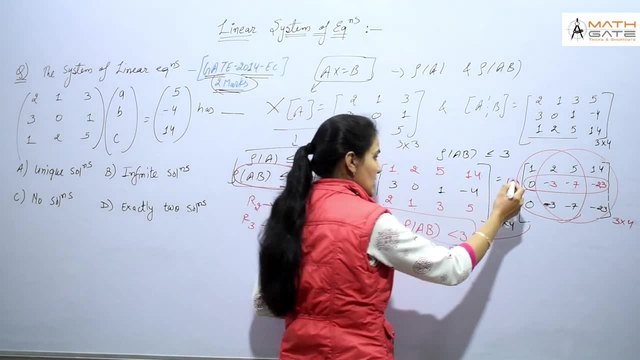 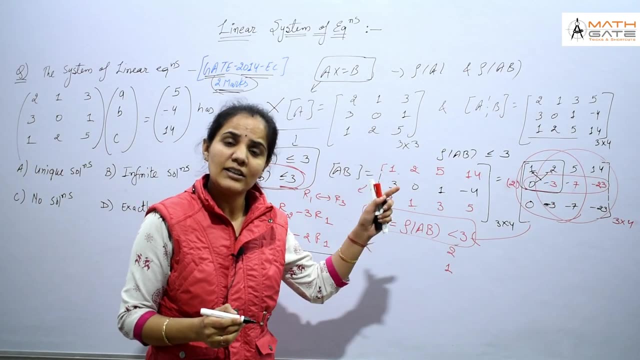 What is it For that? what will we do For that? we will go to the first minor of 2 cross 2.. If we check the first minor of 2 cross 2 in this matrix, then we will get whatever value it is. 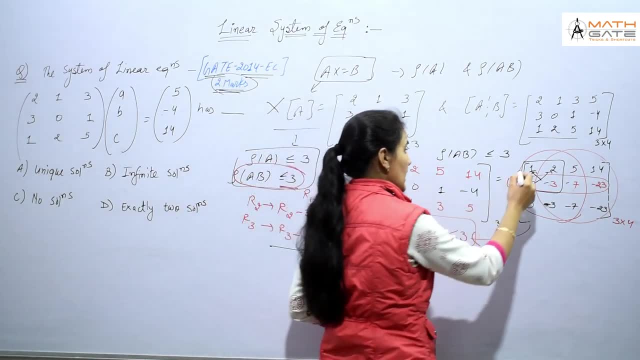 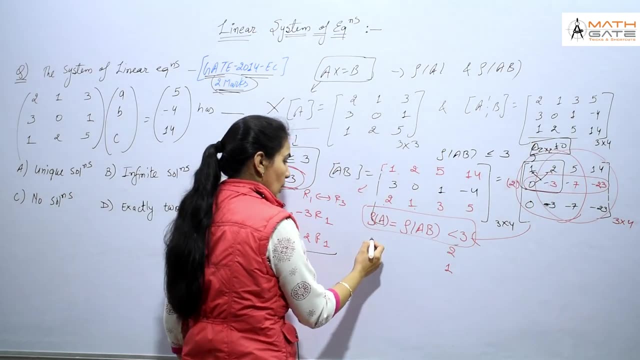 that is equals to non-zero. This non-zero is going to come From here. the value of the minor of 2 cross 2 is going to be students non-zero. If it is non-zero, then you can say clearly: 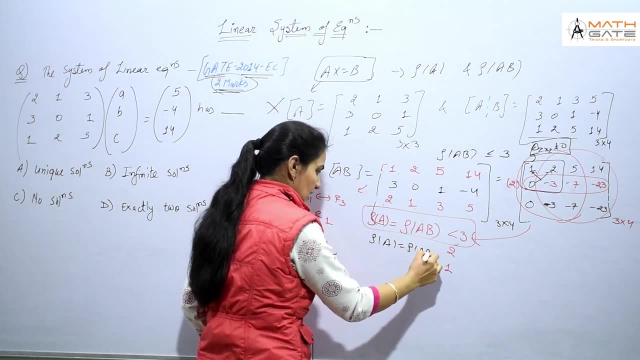 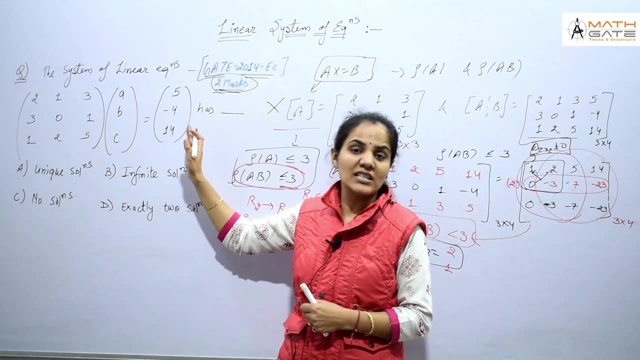 rank of A and rank of AB is equal to what Students? 2. If rank of A and AB- both of them came, 2 came to you. And the number of unknowns in this given question? how many are there? 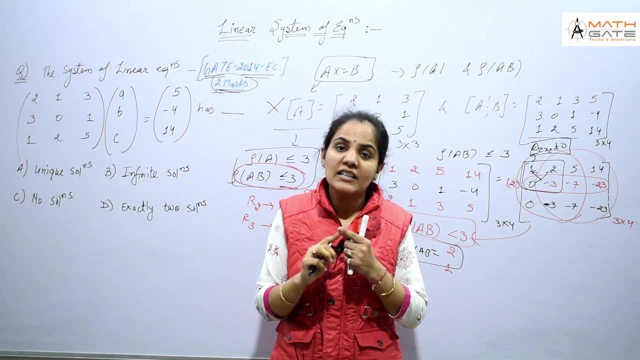 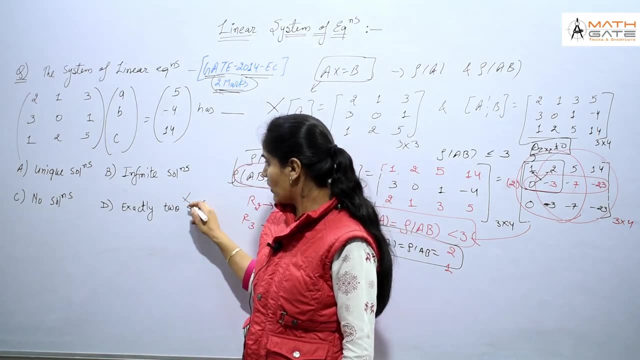 A, B, C, that is equal to 3.. So you understood clearly that the rank that is coming, the rank that is coming to you, what is it? The number of unknowns is less than coming. This means exactly 2 option cannot be there. 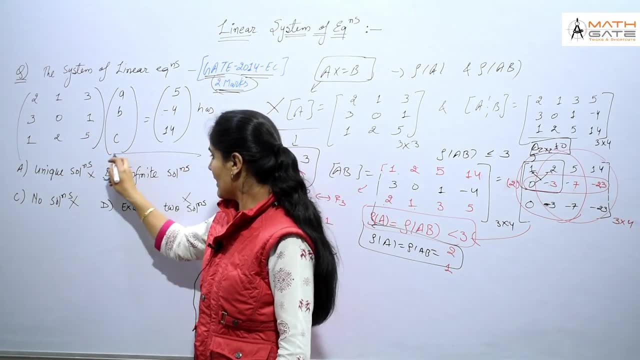 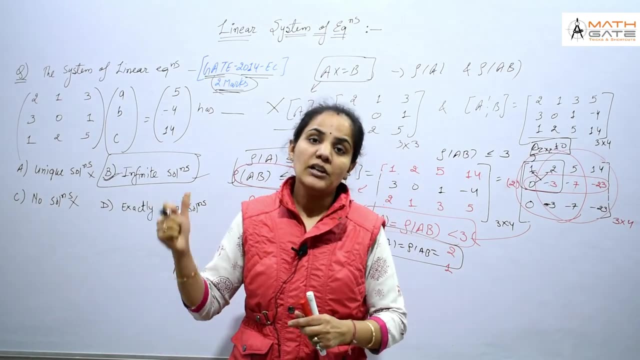 No solution cannot be there, It cannot be unique. What? What is going to happen? Only infinite number of solutions is going to be the answer to this question. It is a very important question because it is a very basic question, If you understand this. 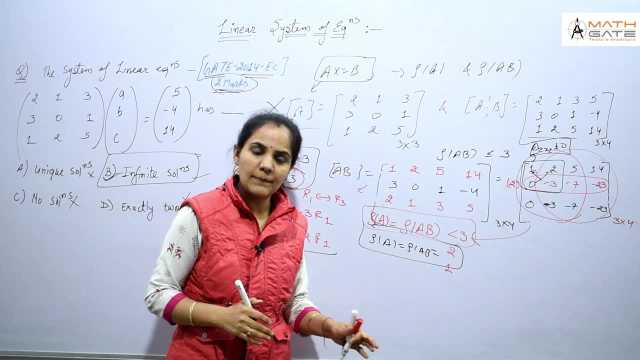 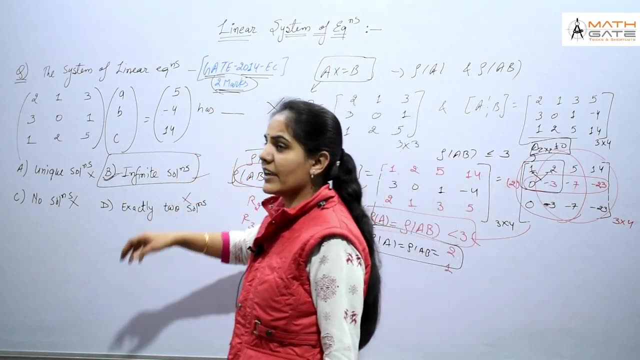 then you can do any question related to this one. You can do any question. Very good and important question. Understand it easily. Okay, let us take a quick revision of this question again In GET 2014,. 2 mark. question has come. 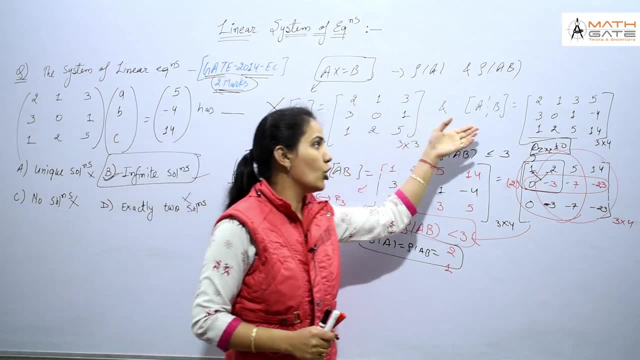 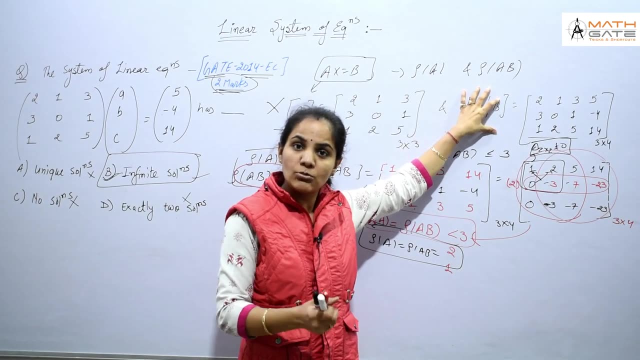 We have this matrix. The value of this matrix A is this, And augmented matrix AB is this: We have not solved matrix A separately. We have taken augmented matrix AB only This augmented matrix will give me the rank of matrix A and matrix AB. 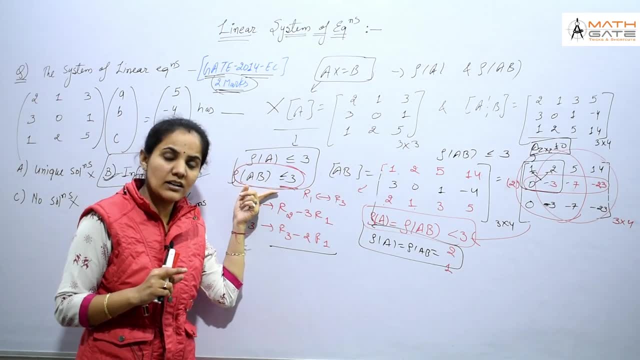 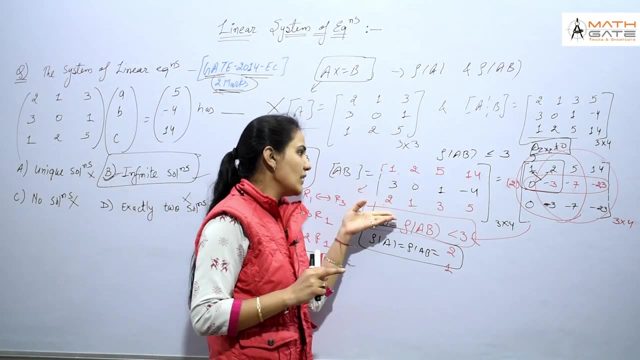 So when I solved for matrix AB then it showed me clearly that rank of AB is less than or equal to 3.. Same with the rank of AB, it will be less than or equal to 3.. So to solve for AB, 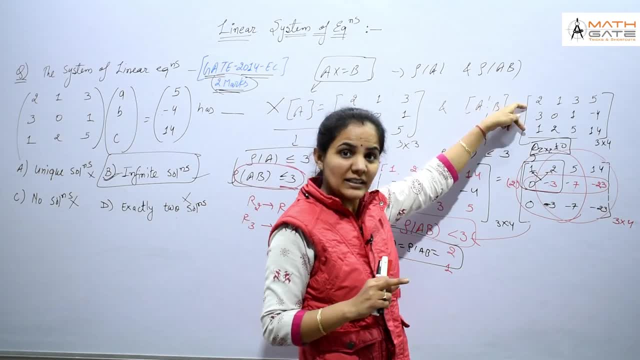 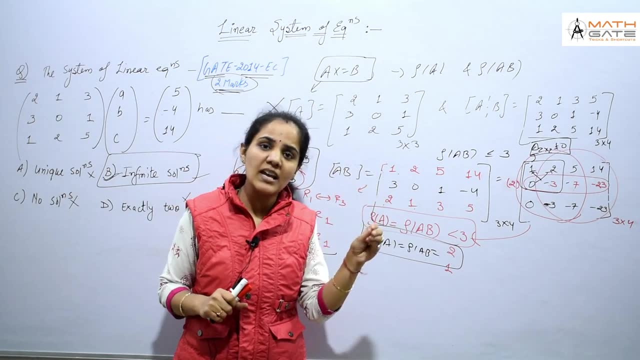 what have you applied? You have applied transformation, You have interchanged this first and third row. We know that if we interchanged row or column, then sign negative comes. But here I do not care about the value, Here I do not care about. 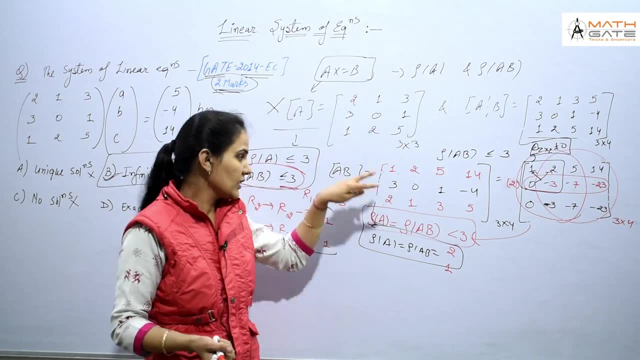 the value of the determinant. So I have made sign negligible. Okay, So here I have interchanged. After that I have applied transformation. Basically I have applied R2 minus 3 R1 and R3 minus 2 R1. 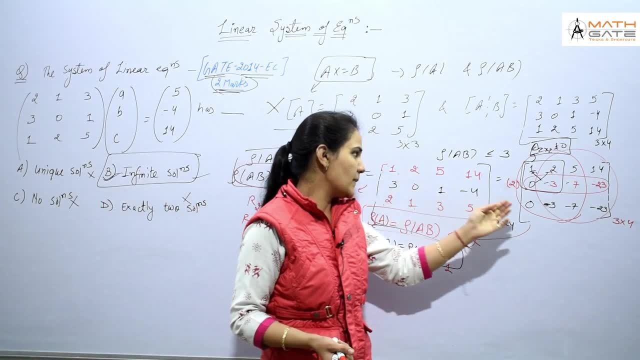 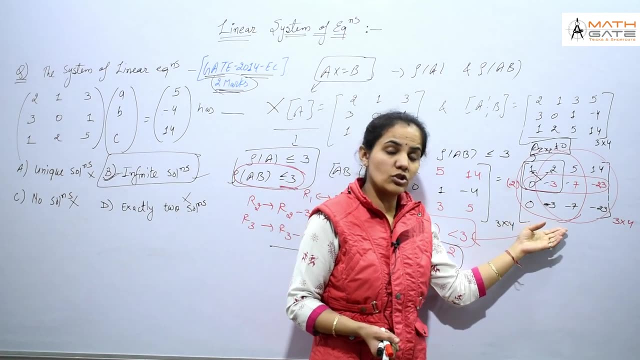 on the place of R3.. Then the matrix that we have made in that matrix. what are the two rows? They are identical. This means all the matrixes of this 3 cross 4, the matrix of this 3 cross 4,. 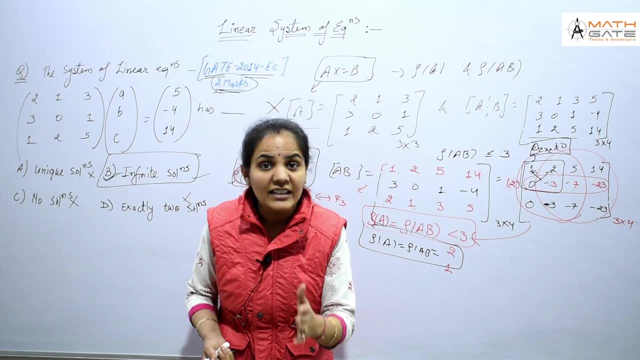 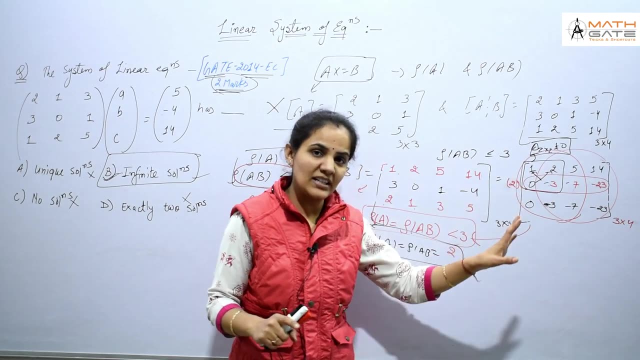 in this, all the minor of 3 cross 3 are going to be made. What will be the determinant of all the minor students? It will be 0.. Okay, Now it will be 0.. It means what has happened is that. 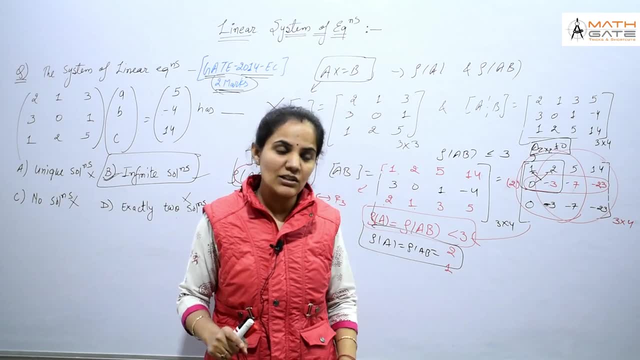 the rank of this given matrix can never be 3.. So what can happen? It can be less than 3.. There are options in less than 3. Either it will be 2 or it will be 1.. So what will you do for 2?? 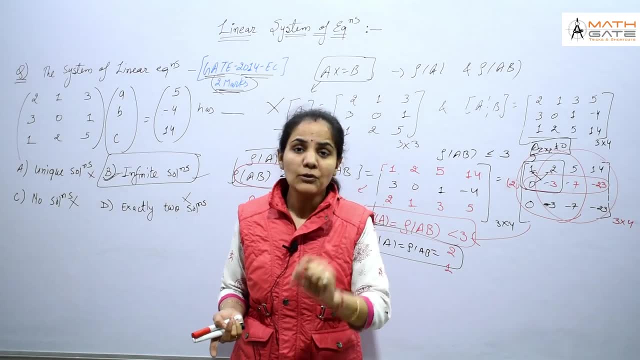 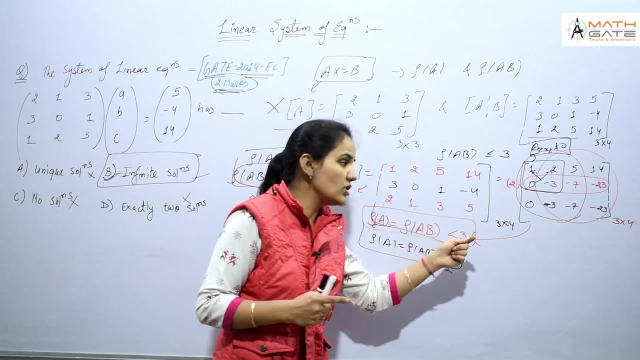 You will check the first minor of 2 cross 2.. You will check the very first minor of 2 cross 2.. And if you got that minor is equal to non-zero, that minor is non-zero, then clearly you can say that. 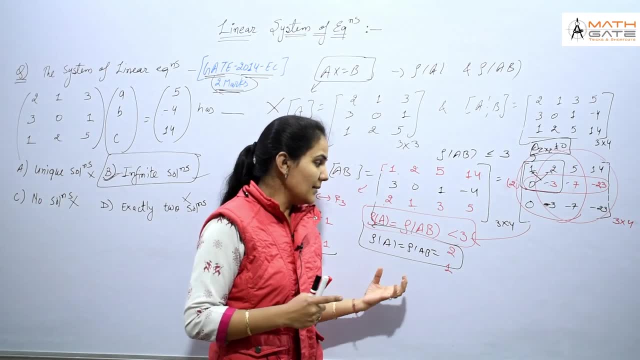 what will be the rank of A and the rank of A? It will be 2.. Okay, If the rank of both of them is 2, and the number of unknowns is 3,, then what will be the solution? Infinite number of solutions. 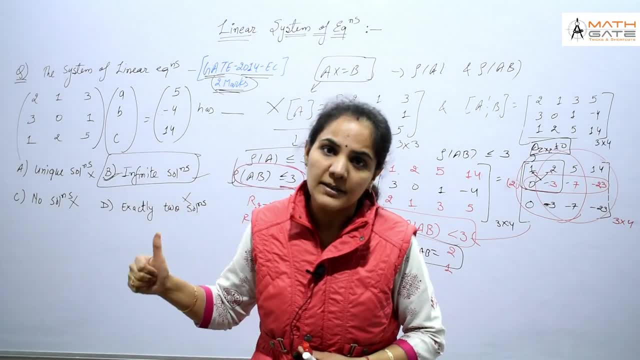 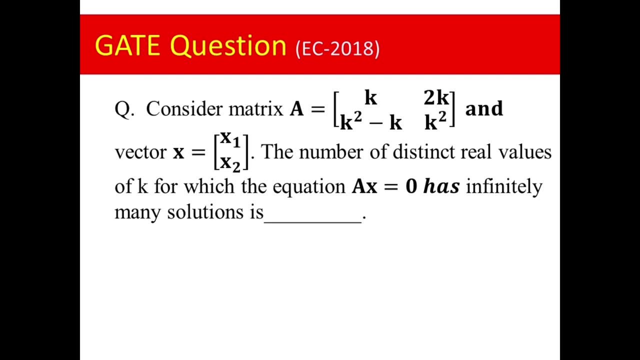 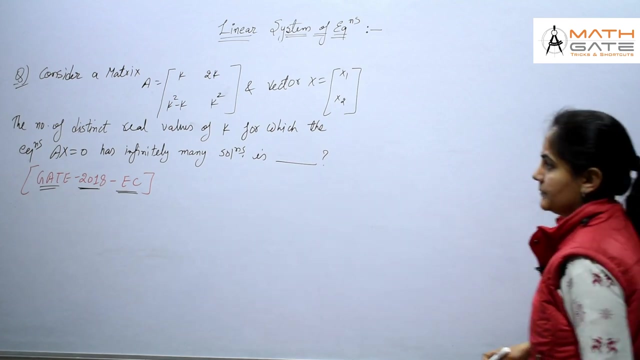 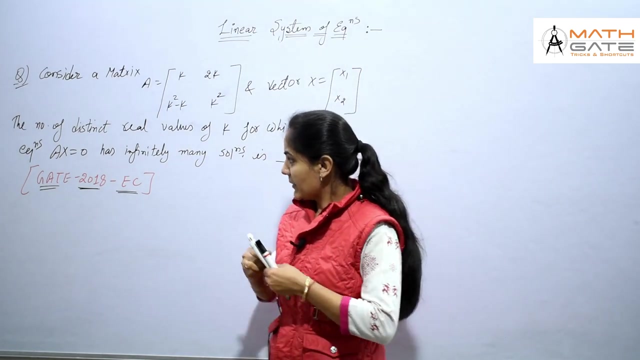 Okay, So the answer for this question is option B. Let us discuss one more question based on Get to the Win. It has come in 18.. Now let us discuss one more question based on linear system of equation, which came in Get to the Win 18. 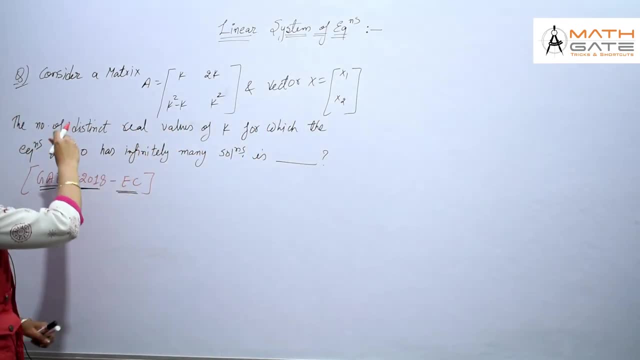 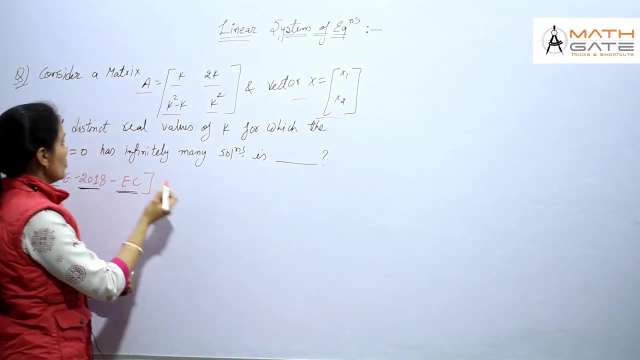 EC branch. Okay, students, Now what is the question? Consider a matrix: A equals to k, 2k k square minus k k square, and vector x is equals to x1- x2: the number of distinct real values of k. number of distinct. 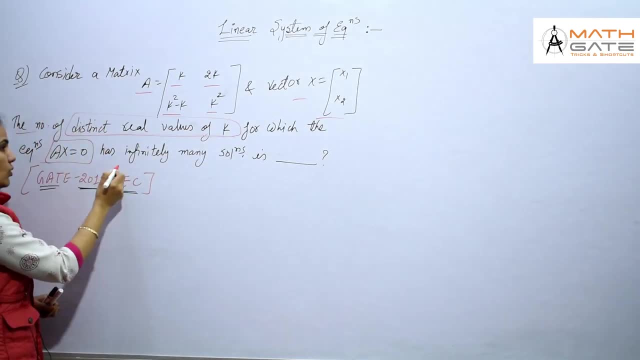 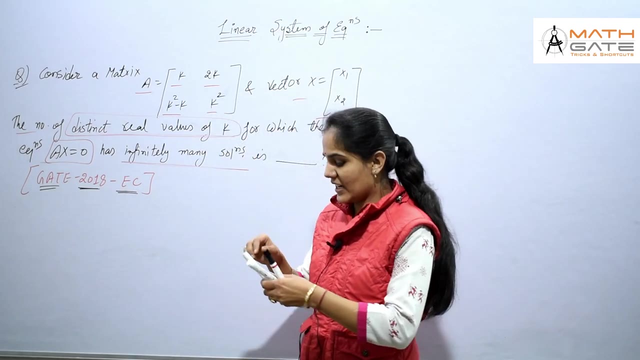 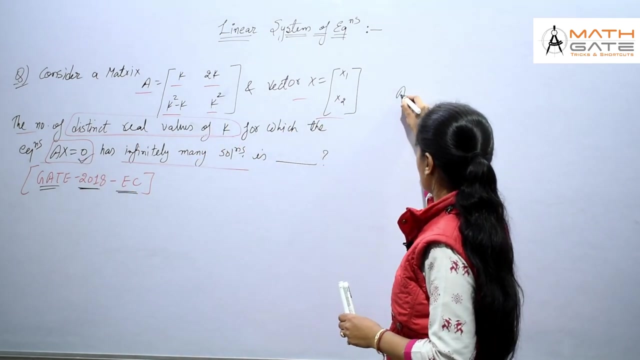 real values of k for which the system x is equals to 0, has infinitely many solutions. It is a very good question, students. It is very clear that the system of equation is a homogeneous system of equation. If this homogeneous system of equation means 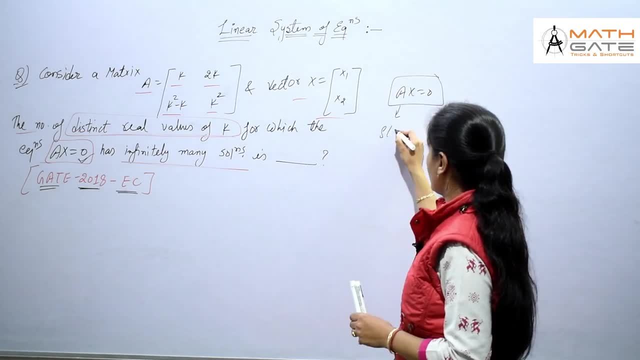 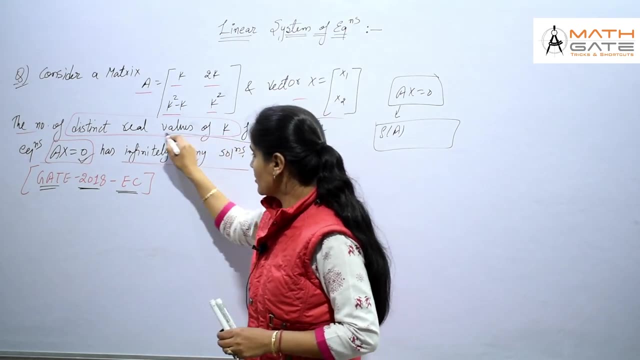 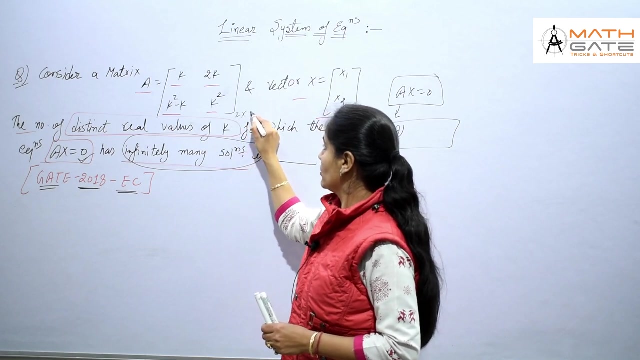 AX is equals to 0. system of equation. it means everything will depend on the rank of matrix A. and it is telling you that. what kind of solution is there in the system? already you have given infinitely many solutions. If in this system matrix is 2 x 2, 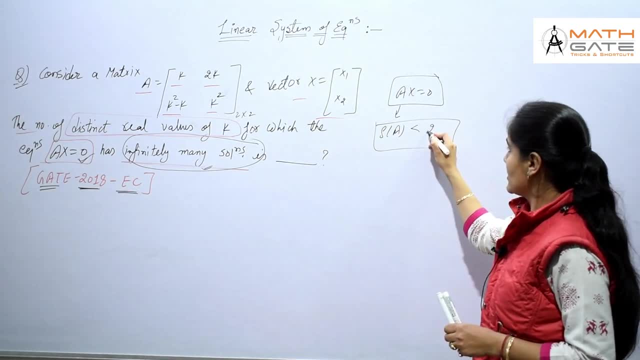 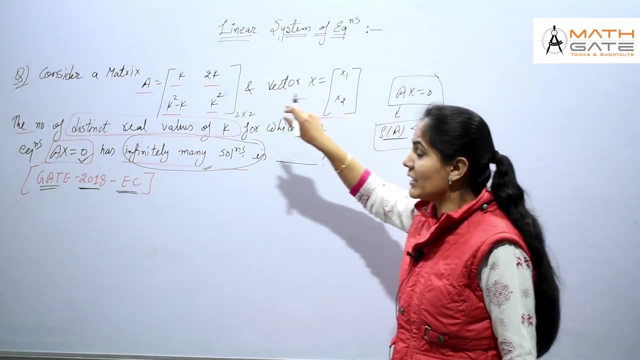 its order is 2 x 2 and it tells you that there are infinitely many. It should be less than 2, because here the number of unknowns is 2 and the number of variables is 2.. So it is clear that the rank of the given matrix A cannot be 2 at all. 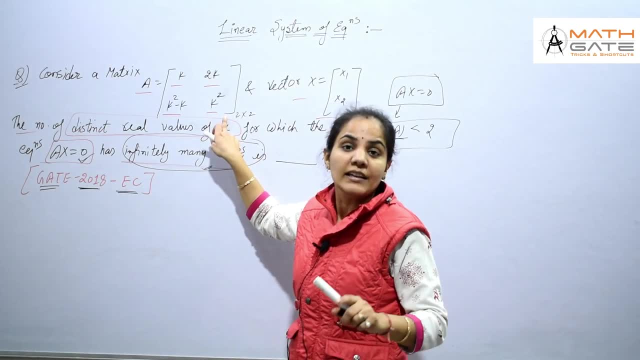 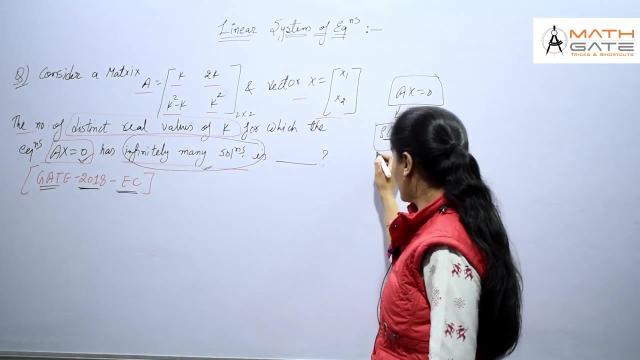 If the rank of the matrix A of 2 x 2 cannot be 2, then it is clear that what will happen to the determinant of the matrix A of 2 x 2? The determinant of the matrix A of 2 x 2 will have to be 0. 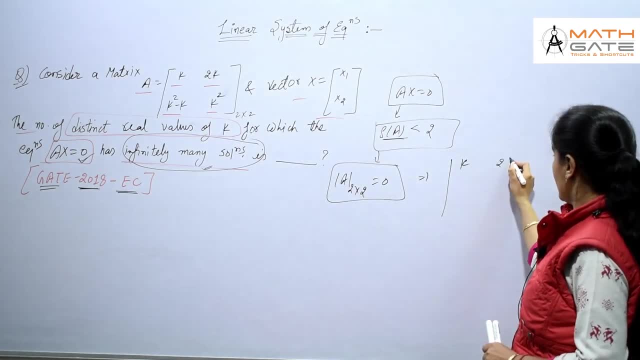 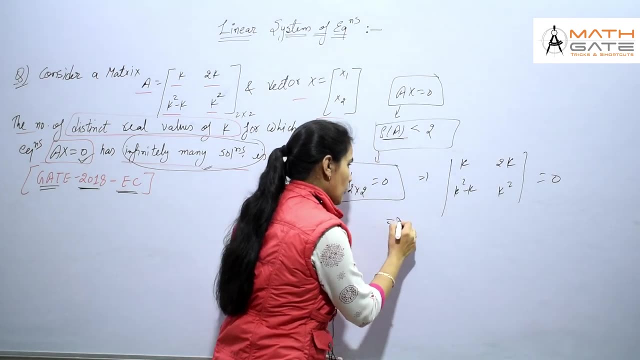 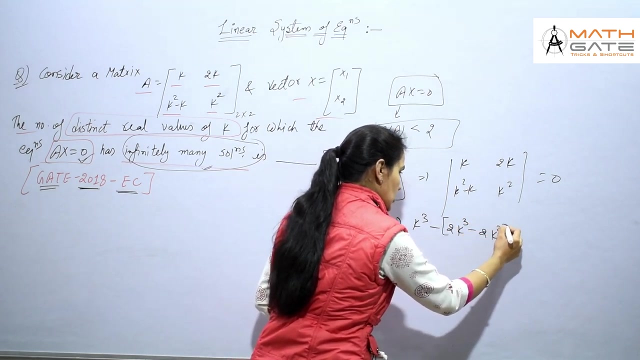 So what you have to do is simply put the determinant of the matrix A of 2 x 2 as 0. Then what you will get? You will get some values. You will get: k cube minus 2k cube, or minus 2k square, is equal to 0.. 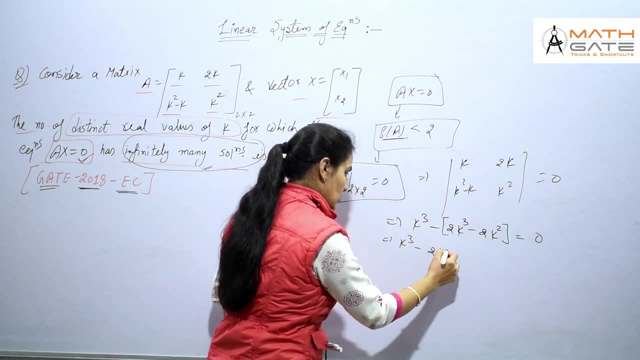 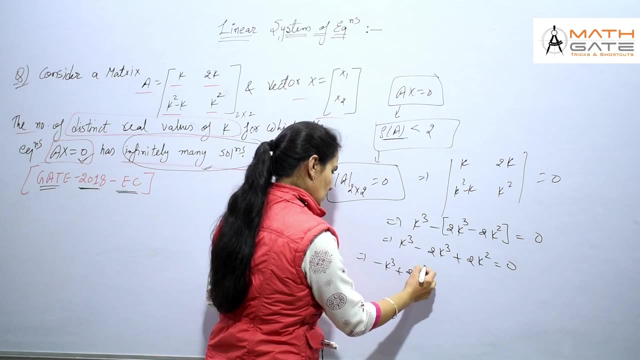 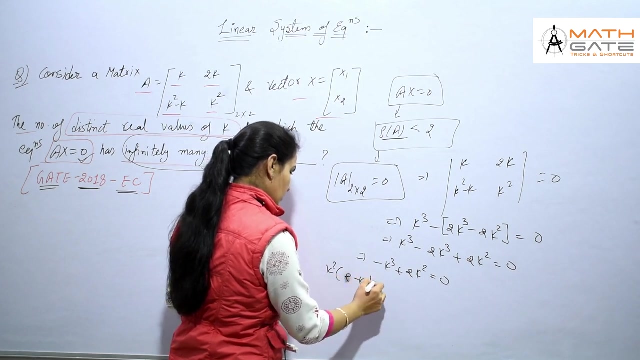 Let us simplify it a little. Then you will get k cube minus 2k cube plus 2k square is equal to 0. Means you will get minus k cube plus 2k square is equal to 0. And you can say k square. if you take it commonly, then you will get what 2 minus k is equal to 0.. 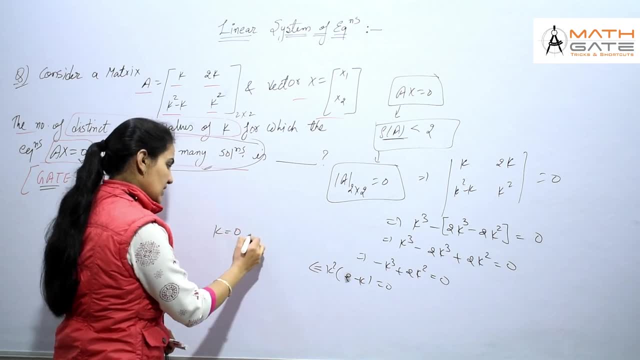 This means you can see clearly that the value of k will come from here: 0, 0.. And what will come? Students 2 will come. I am asking you in the question how many values of k will come which will be distinct? 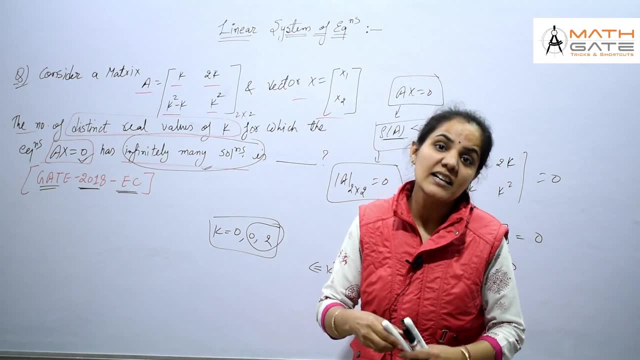 So how many distinct values are coming? Only two are coming. Which ones are coming? 0 and 2 are coming. So how many distinct values have you got here? The different values of k, that is equal to what? 2.. So how many distinct values have you got here? The different values of k, that is equal to what 2.. So how many distinct values have you got here? The different values of k, that is equal to what 2..